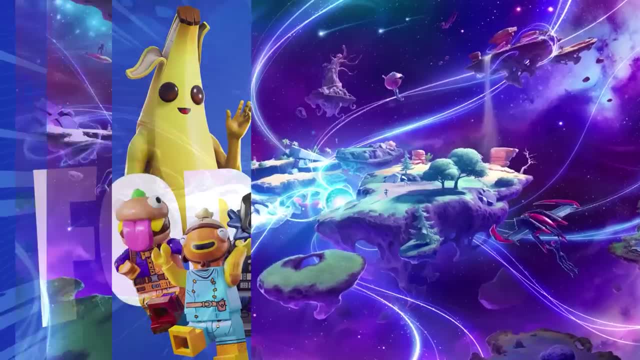 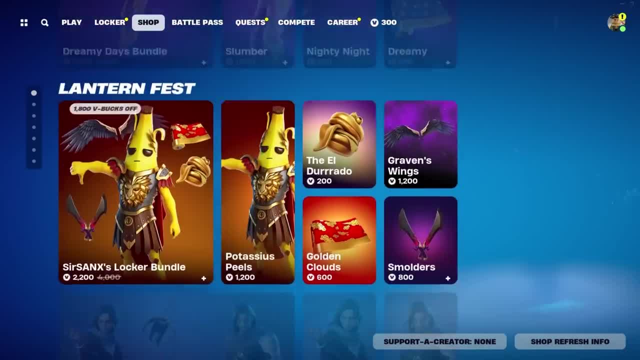 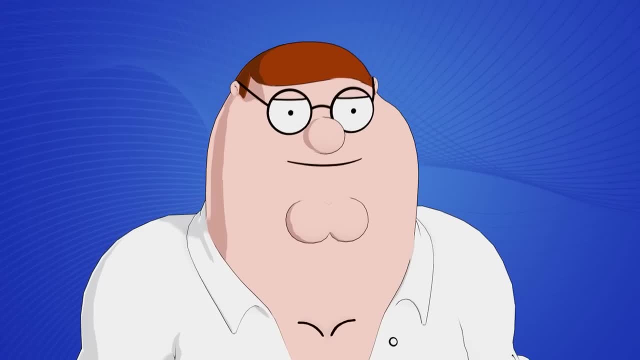 and amazing Game Theory. Was it the ever-growing and amazing Game Theory? Was it the seemingly infinite list of microtransactions? No, it was that. in Chapter 5, Season 1, they added Peter freaking Griffin, And this Peter is putting the cut in cutaway gags. Now this isn't without. 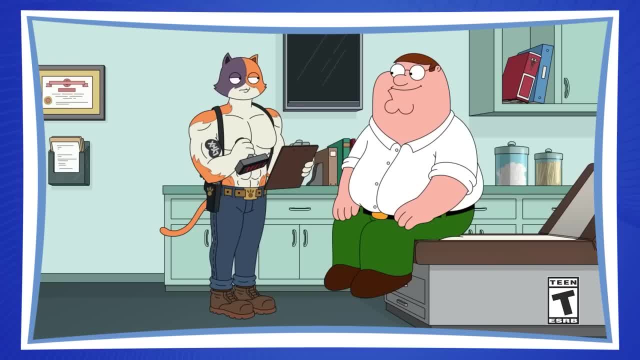 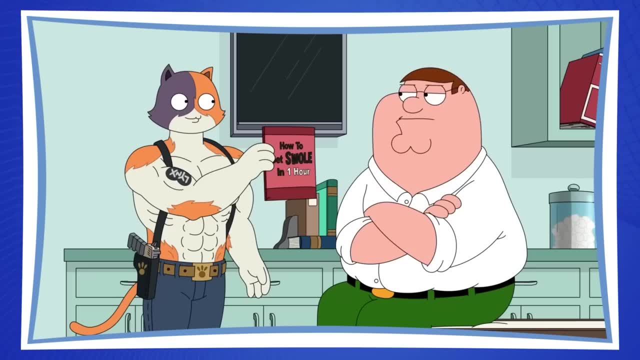 explanation. In the video announcing his addition to the game, we see Peter at the doctor's office getting a physical from Fortnite's resident swellcat Meowcicles- Meowcicles- How is that word pronounced? Oh no, Getting a physical from Fortnite's resident swellcat Meowcicles, Peter. 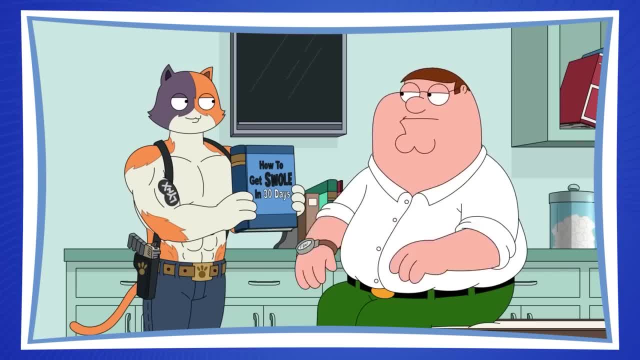 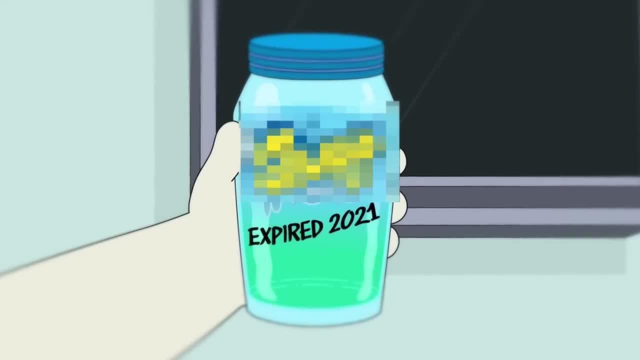 makes it quite clear that he's trying to get jacked, but he's not actually willing to put in any work. So instead, Meowcicles decides to give Peter a jar of something and boom- instant muscles. What was in that jar that helped Peter go from family guy to fitness bro? None. 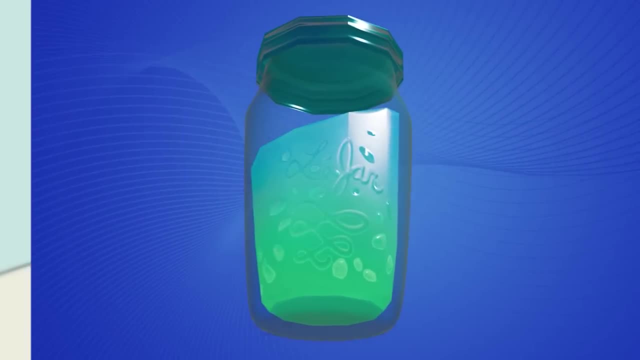 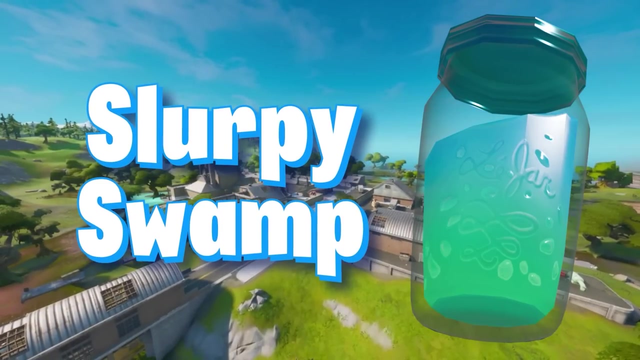 other than Fortnite's iconic Slurp Juice. This slurpy goodness was a consumable item in Fortnite that used to heal quite a bit of health back in the day. It was created by Slurp Co in the aptly named Slurpy Swamp. Over the years, Slurp Juice has been added and removed and added again. 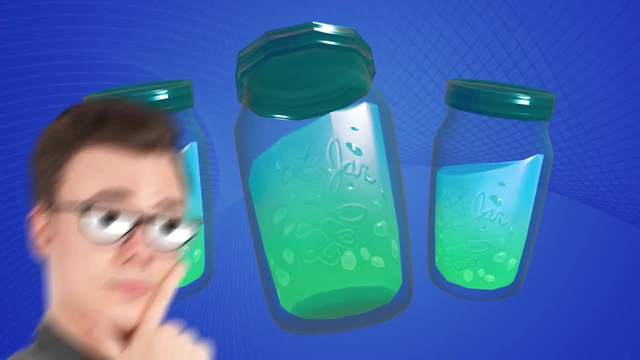 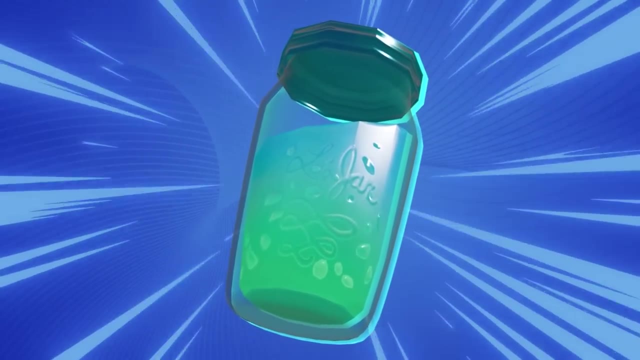 but it still remains one of Fortnite's most iconic and beloved items. But the only thing I could think of when I saw Peter down that juice is: could something like this actually exist? I mean, Slurp Juice seems to pack a pretty powerful punch. 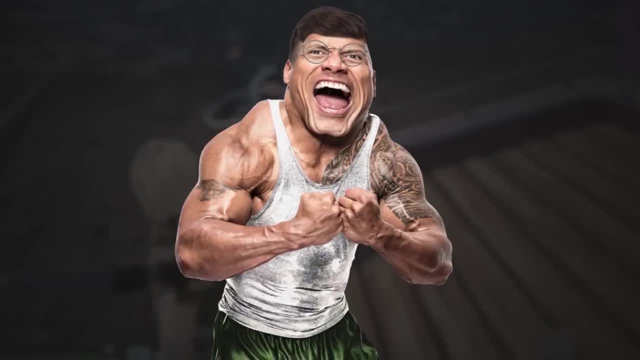 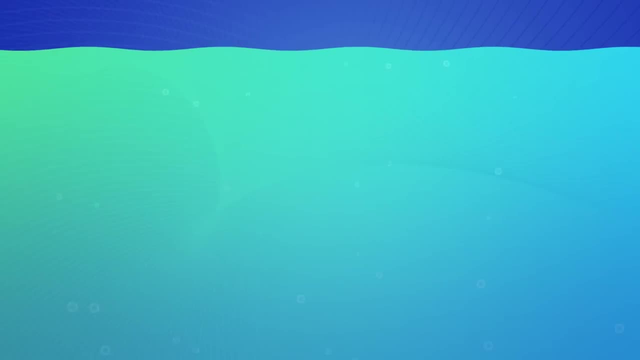 Not only does it heal all wounds, but it also can turn Peter Griffin into Dwayne the Rock Johnson. Could a juice help heal you and grow your muscles without you having to lift a finger? The answer, as it turns out, is an unequivocal yes. After hours of research, I think I may have discovered: 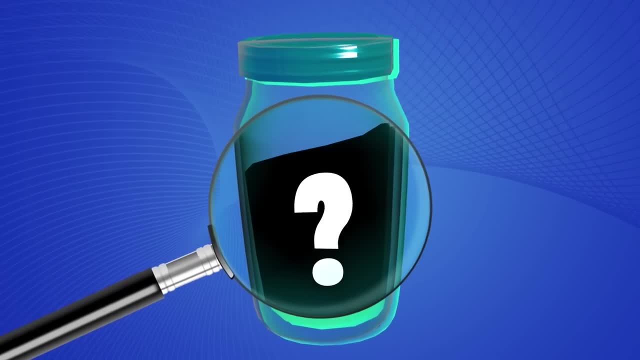 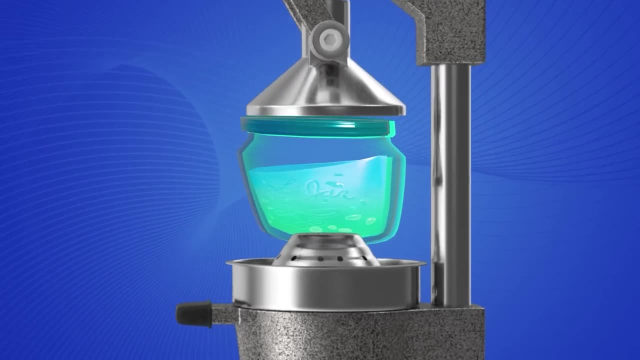 the secret ingredient that makes Slurp Juice so slurpy, and it's something that you might find in your local pharmacy sooner than you'd think. Grab your mason jars and juice presses. loyal theorists: Time to squeeze every bit of science out of this six-year-old item. 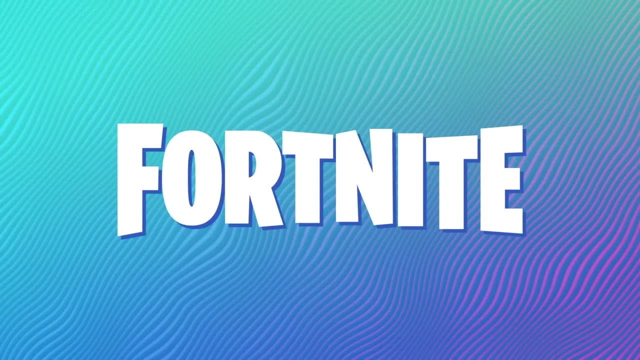 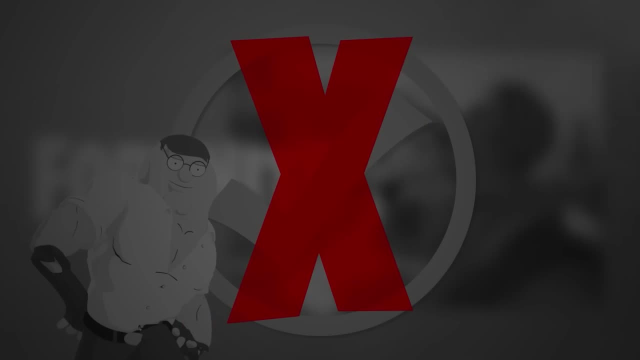 To kickstart our slurpy investigation, I of course turn to the game itself. Does it give us any indication of what Slurp Juice might be? It does, but not in the battle royale. Instead, the answer actually comes from the newest addition to the Fortnite family: Lego Fortnite. Lego Fortnite is. 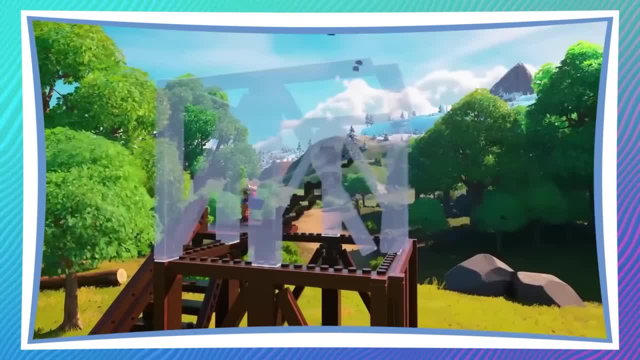 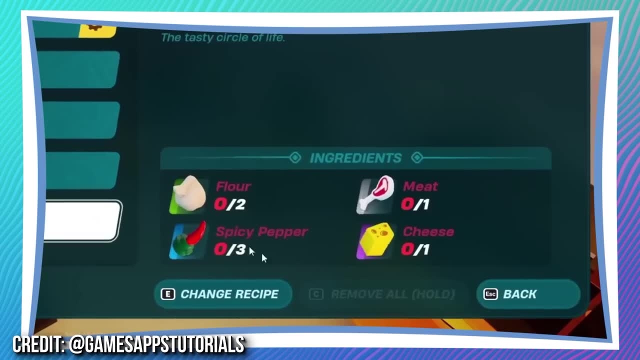 an open-world survival crafting game that converts everything into the lovable Lego brick style. Huh, wonder how Mojang feels about that. Anyway, because of that, crafting Lego Fortnite allows you to take raw ingredients and turn them into consumable items, including Slurp Juice, which only requires. 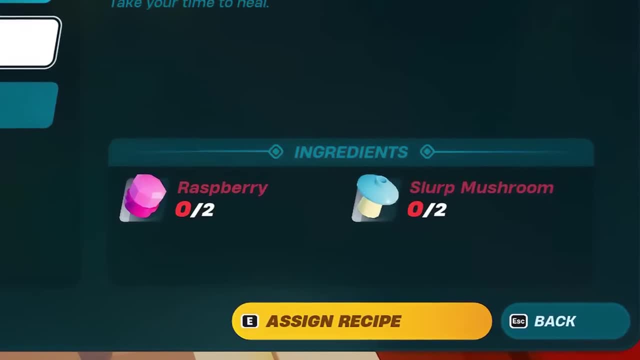 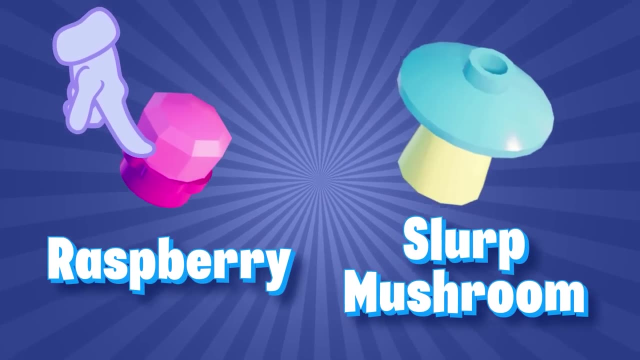 two simple ingredients: Raspberries and Slurp Mushrooms. There you have it theory over. we figured out what Slurp Juice is, But obviously we're not done, because while we have the ingredients, we need to see whether they would actually achieve what the game suggests. So it's. 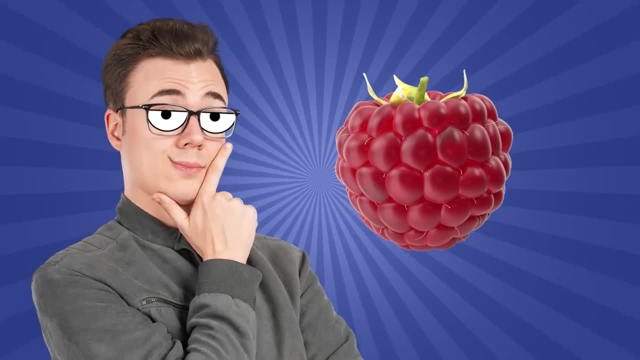 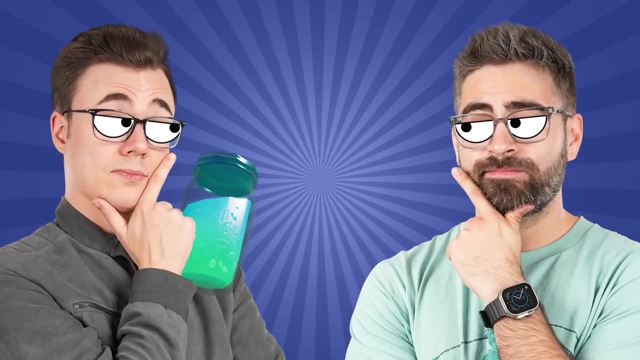 time for some good old-fashioned food science. For starters, raspberries are-. Uh, what do you think you're doing? Oh, it's Santi. What does it look like I'm doing? I'm about to explain the science of a video game. 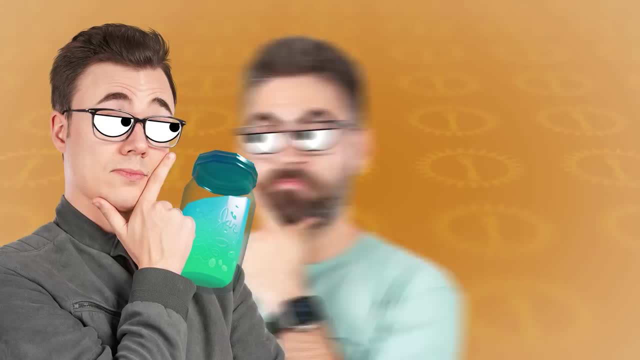 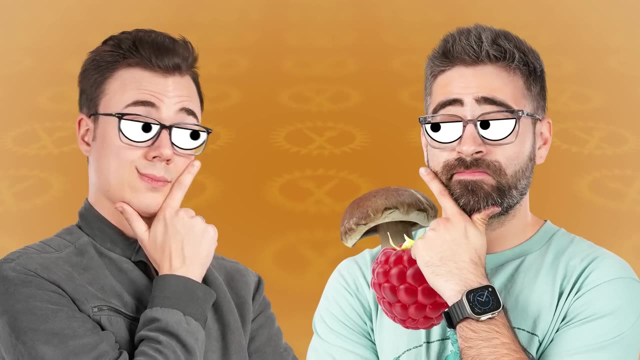 item. What it looks like you're doing is trying to steal my thing. I'm the food theory guy. Tell you what. why don't you tell the audience about the nutritional value of raspberries and mushrooms? and I'll chime in to talk about how it helps us solve our in-game mystery. 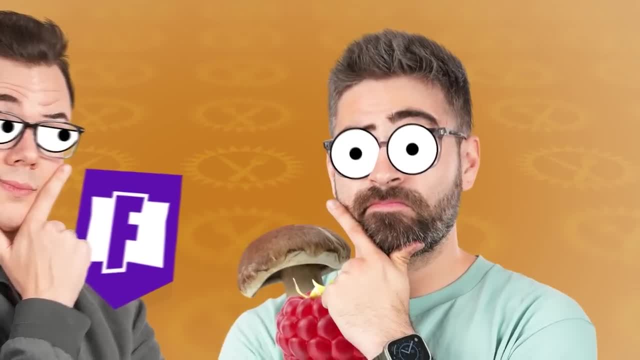 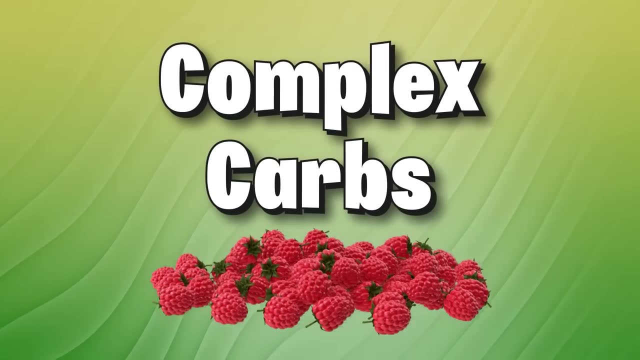 You mean like work together. I guess I could give that a try. Raspberries are actually a great ingredient to have in an athlete's juice. They're an excellent source of complex carbohydrates, supplying your body with a sustained energy source. Raspberries also contain beta-carotene. 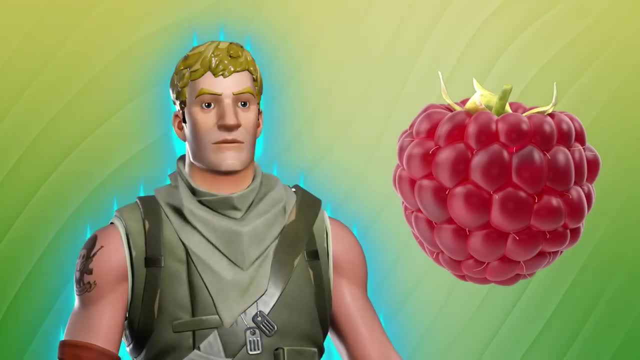 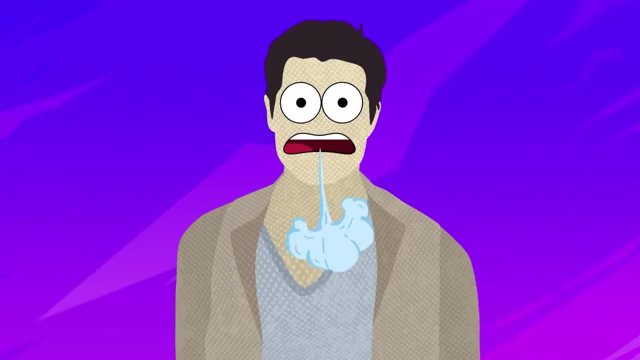 which can improve eyesight. So with raspberries, a player can push for longer while also no-scoping the competition. Exactly, Raspberries are also chock-full of antioxidants like vitamin C and E. You see, every time you breathe, your body produces what are known as free radicals. Free radicals end up. 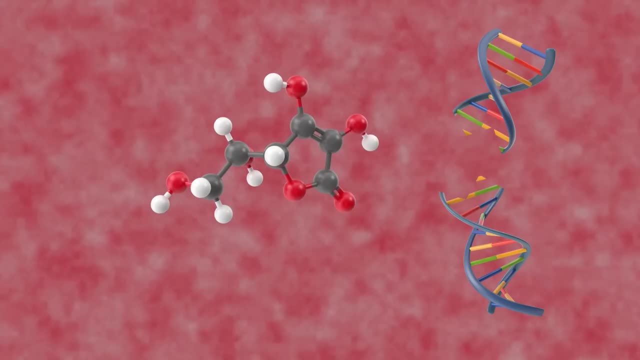 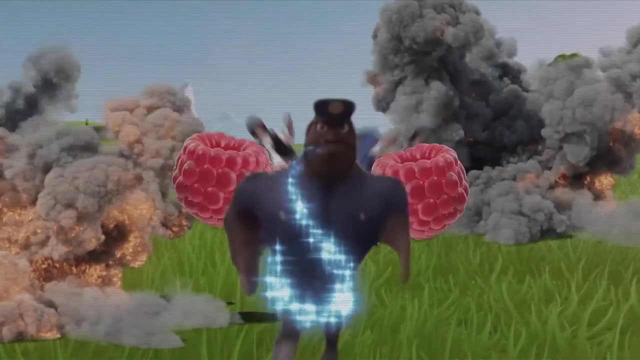 damaging your DNA and tissues. Antioxidants are able to neutralize those free radicals. So if a person is running around an island trying to survive, they would produce a lot of free radicals, right, But the antioxidants in the raspberries would help to heal them from. 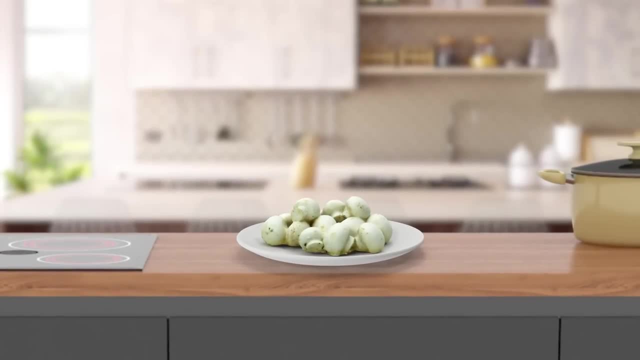 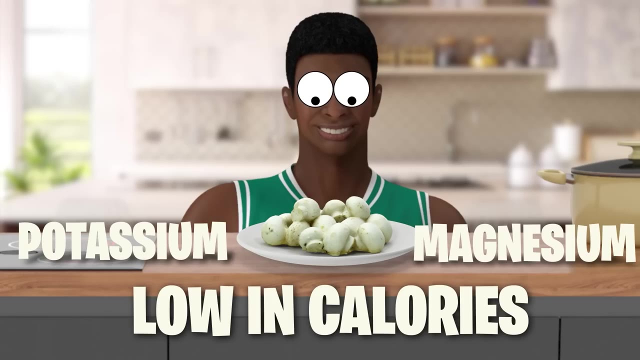 those effects, so to speak, Now you're cooking. Mushrooms are another ingredient that athletes have been gravitating to lately. They're low in calories, they contain minerals like potassium and magnesium that help muscle function, and they're a pretty decent source of protein If you're looking for a non-meat alternative for. 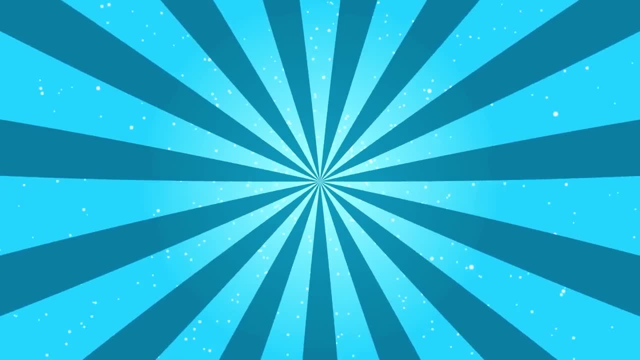 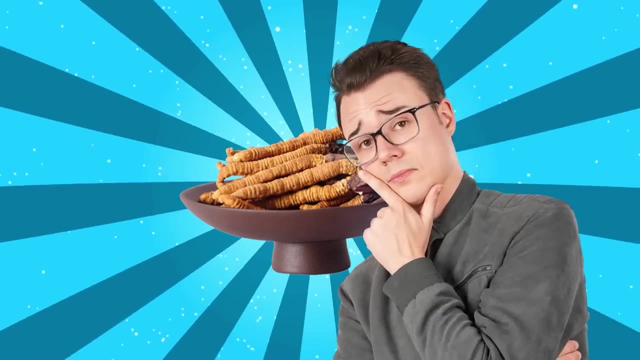 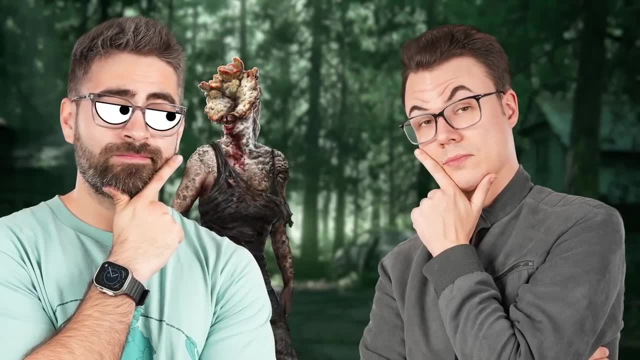 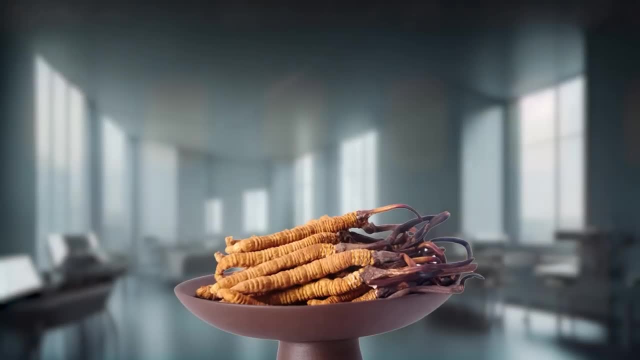 zombie outbreak in The Last of Us. Well, yes, it does share the same name, but it doesn't quite work that way in real life. Cordyceps have been traditional Chinese medicine for centuries, but more modern science research has shown that. 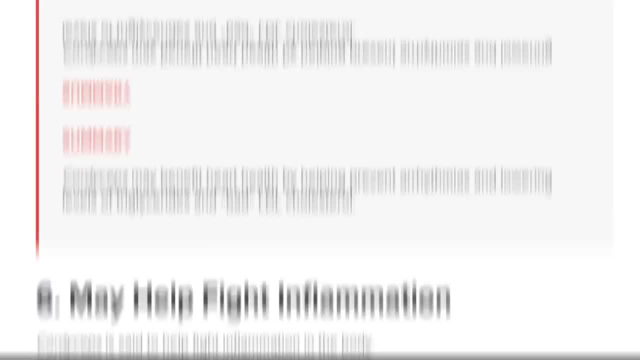 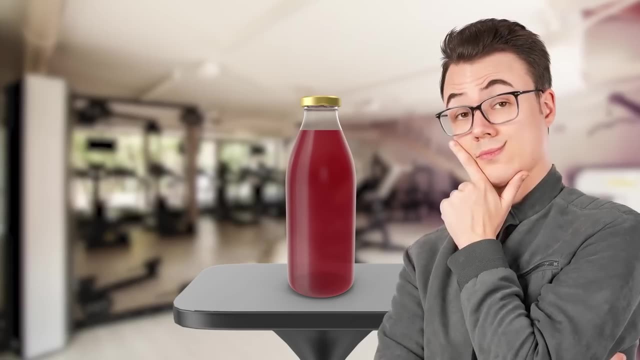 along with the muscle building properties, Cordyceps can boost exercise performance and fight inflammation. All in all, I think that having a raspberry and mushroom juice could end up being the perfect combination for a nice post-workout drink. Wow, I guess. 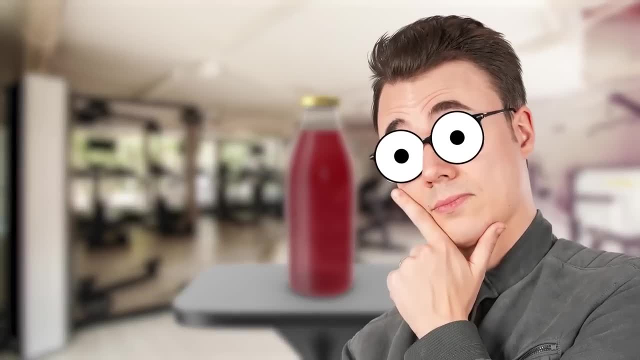 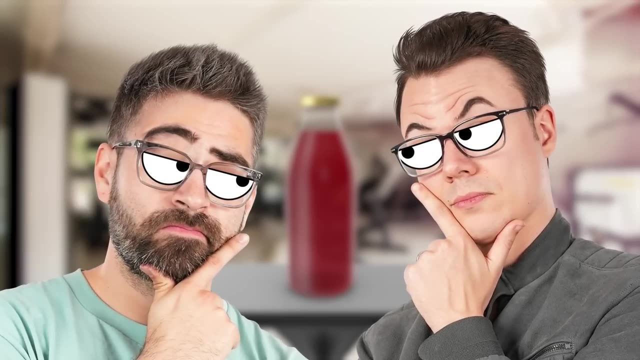 Fortnite really was onto something. Maybe this episode is just that simple. Wait, did you say post-workout? Yeah, I mean you can drink all the nutritious stuff you want, but you're not going to gain any muscle mass or improve your fitness without working out. 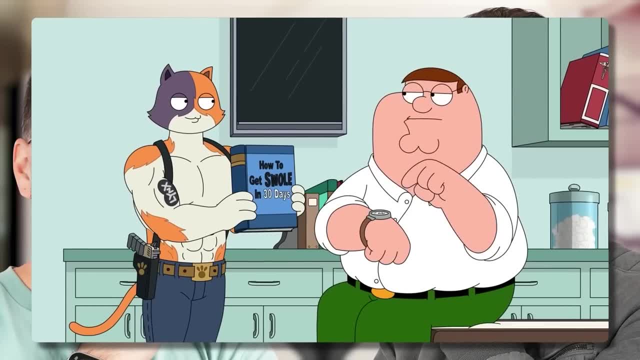 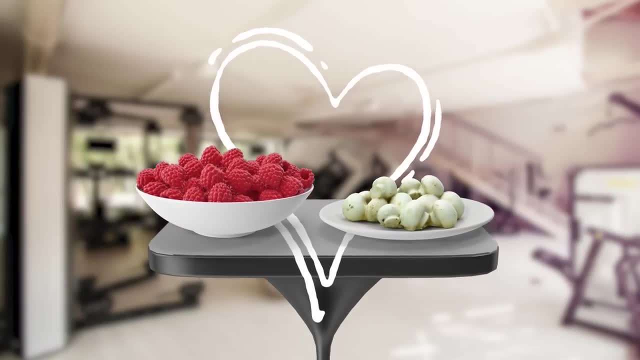 at least a little bit, But that's exactly what happens. Pia rejects the 30 day, one hour workout plan, Which means, while raspberries and mushrooms sound like a perfect fit, we need something that's going to work without having to exercise. So 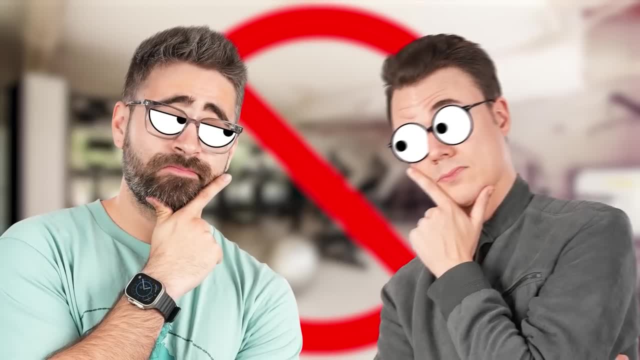 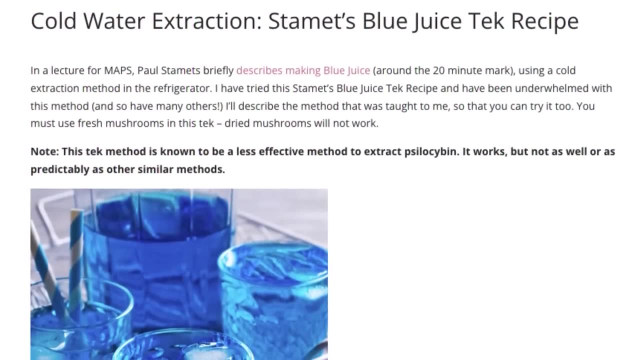 all the research I just did was totally useless. Not useless, Actually, yeah, kinda Okay. well, maybe he's just hallucinating. You can turn magic mushrooms into a psychedelic juice with a suspiciously light blue colour that looks just like slurp juice. 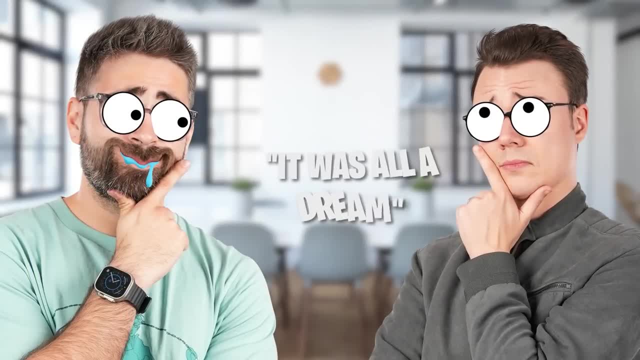 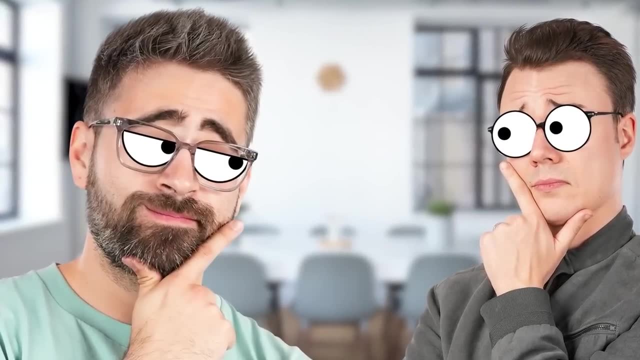 Are you seriously suggesting that I go with? it was all a dream, I uh. yeah, I guess you're right. Well, at least I got to do one of my other favourite things: Waste your time. Bye Ugh that guy. But what he doesn't know is that, thanks to today's sponsor, AFK Journey, 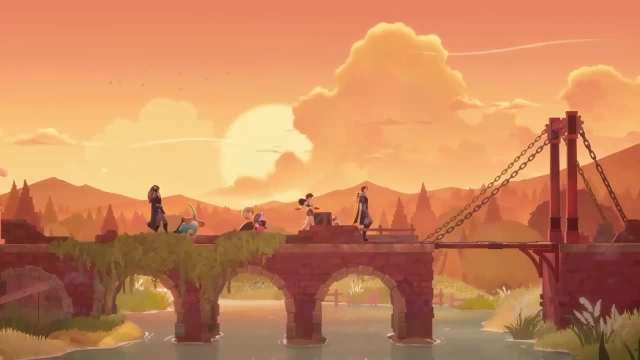 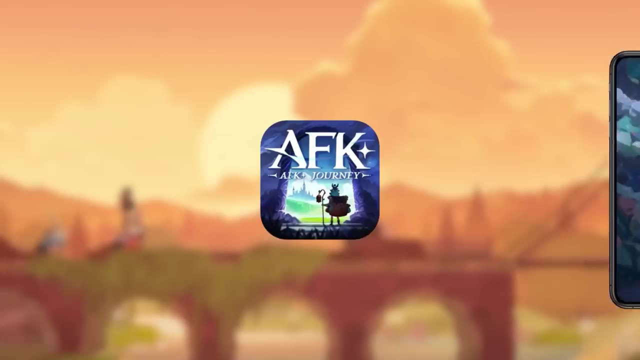 while he thinks he was wasting my time, I've actually been levelling up, growing my resources and gaining some pretty cool rewards, all without having to even open up the game. He'll never know, But what you need to know is that AFK Journey is the latest game from the creators of AFK Arena. 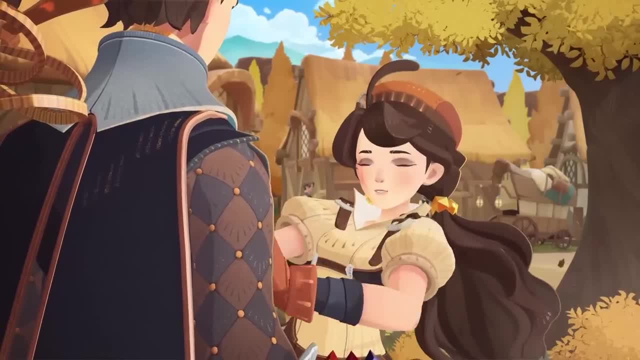 where you get to play as Merlin the Wizard, as you reunite with your favourite heroes from the previous game. And who doesn't want to play AFK Journey? Well, that's what I'm here to tell you. And who doesn't want to play AFK Journey? Well, that's what I'm here to tell you. And who doesn't want? 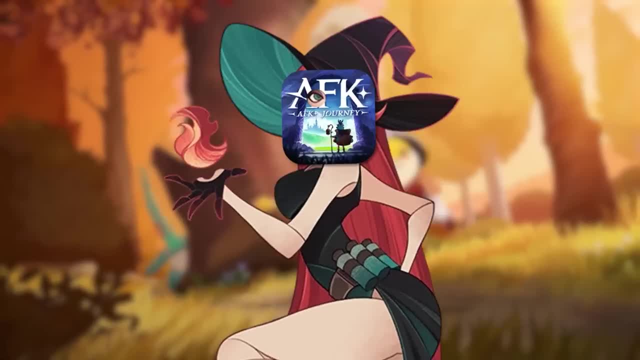 to play AFK Journey. Well, that's what I'm here to tell you. And who doesn't want to be a wizard? But don't worry, the game isn't just a re-skim with a couple of new dance moves: AFK Journey. 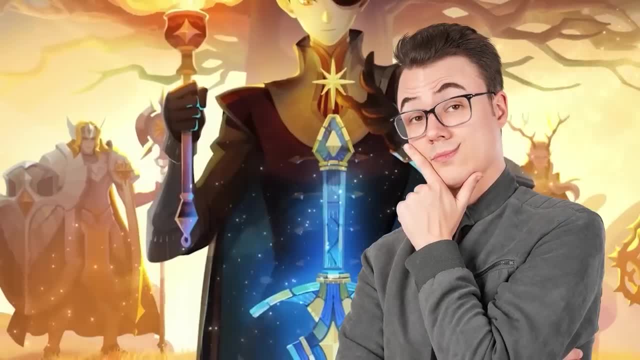 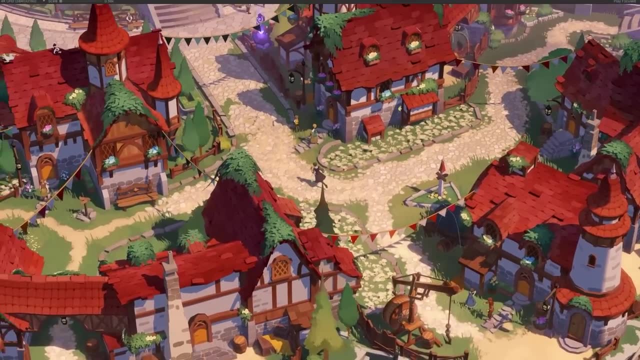 focuses heavily on fantasy RPG elements, And I love me a good RPG, so I was hooked. Can you really blame me? Just look at this thing. The map is huge, which means there's so much to explore, And the world itself is stunning, Whether it's the Golden Wheat Shire or the 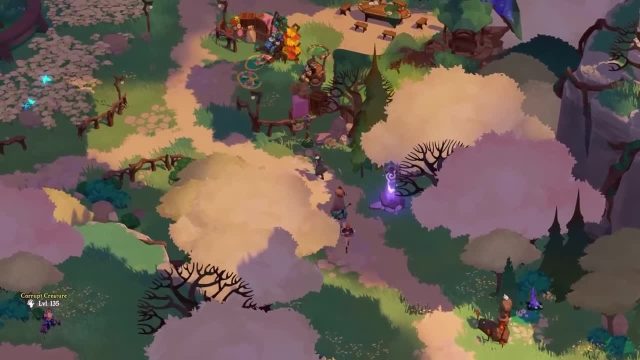 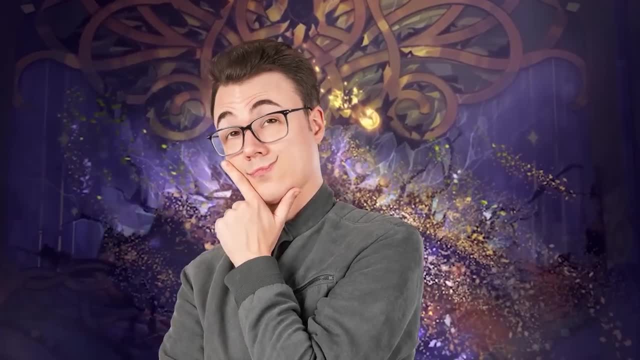 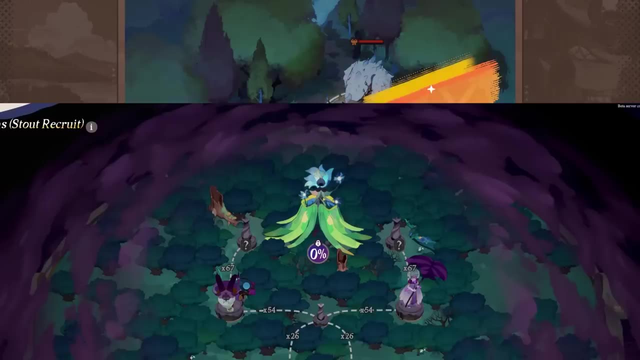 going to lie, And you know how we love that here at Theorist. And what's great is that you and I can lore hunt together, Because AFK Journey allows you to make your own guilds and team up with your friends to take on dungeons, play minigames and explore the vast map faster to help find. 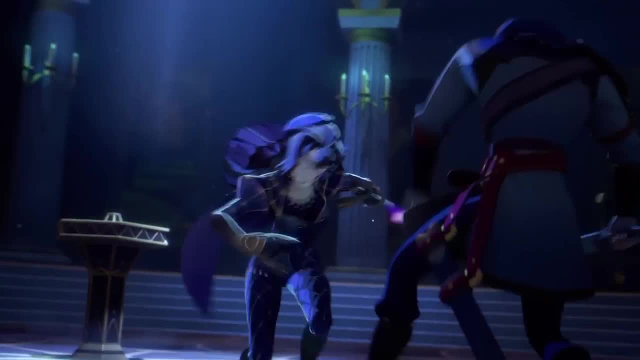 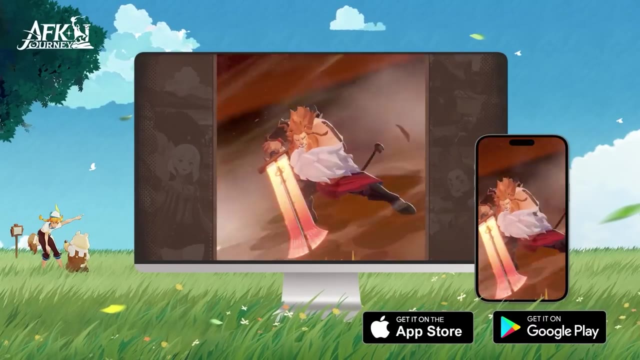 that aforementioned lore. So if you'd like to join the Theorist Guild and help me out, you can head on down to the description and download the game today. It's available on iOS, Android and if you'd prefer to play on a bigger screen, you can now go to the official website. 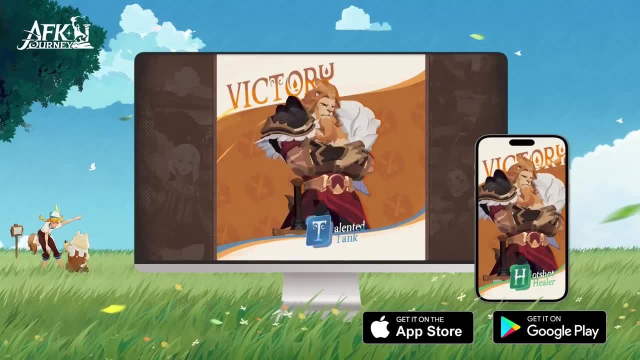 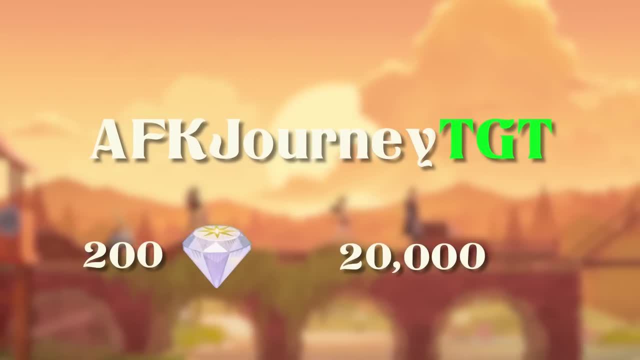 and play it on your PC. Where are my PC? Master Race at Plus, if you use my CD key AFK Journey, TGT, TGT, as in The Game Theorists, you can get your hands on 200 diamonds and 20,000 gold coins. 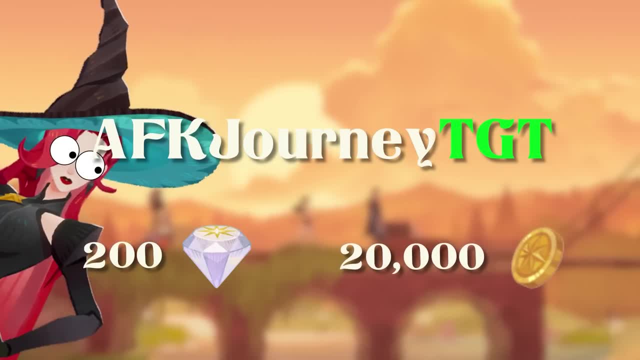 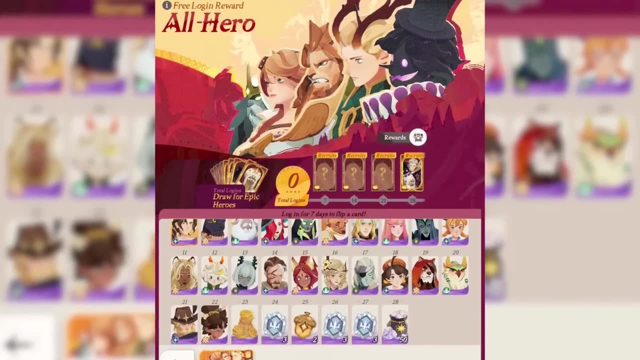 to spend in-game. Though you're not going to be spending any of that on heroes because, as part of AFK Journey's official release, they are offering 40 heroes for free, including epic heroes, Meaning you can really diversify your strategies and customize the experience to suit. 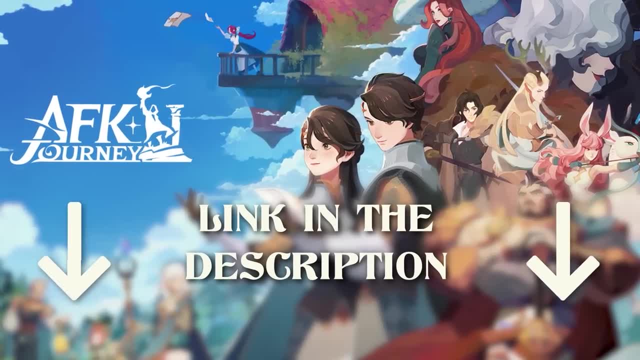 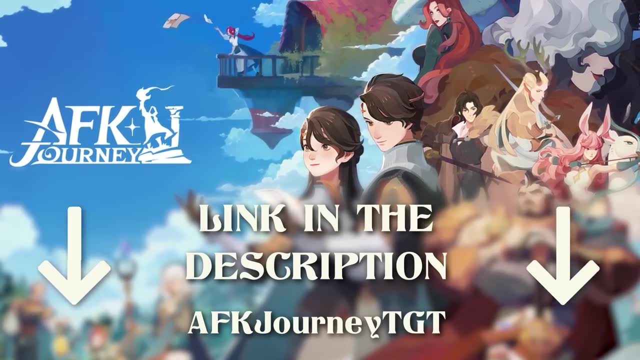 you. So, for all those awesome rewards, click that link in the description and use the code AFKJOURNEYTGT and begin your AFK Journey today. But for now, I shall see you in the next video. For now, I should probably get back to my own journey and figure out what is in this Slurp Juice. 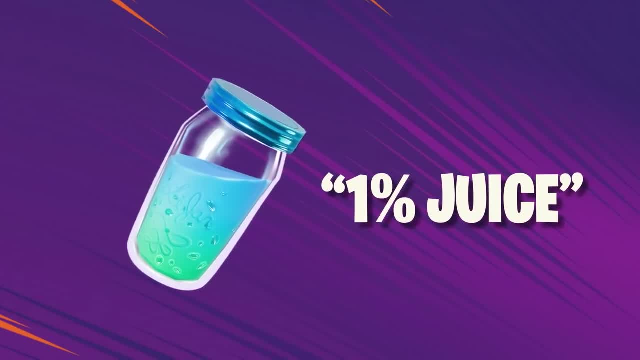 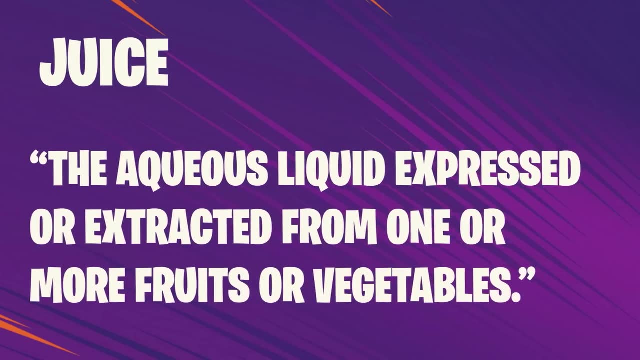 According to the game, Slurp Juice contains, quote- 1% juice and, according to the FDA, juice is defined as the aqueous liquid expressed or extracted from one or more fruits or vegetables. So raspberries and mushrooms are likely part of this concoction, but what on earth is the other? 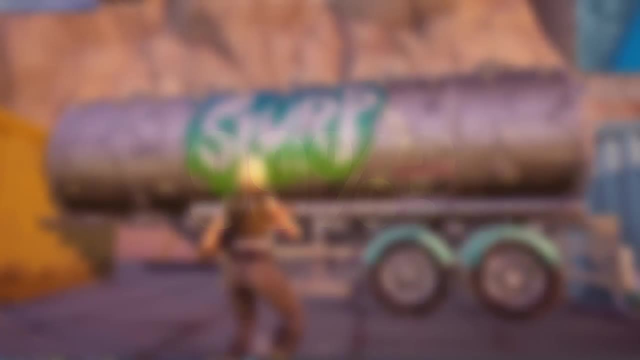 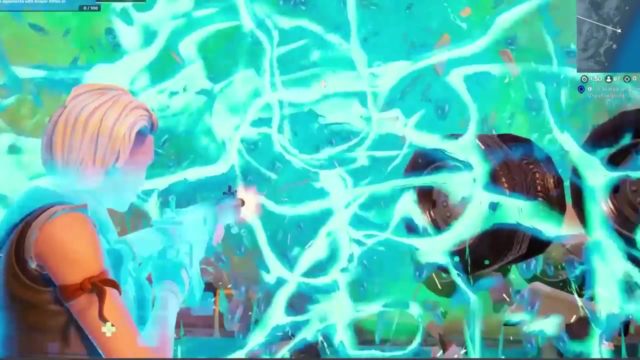 99%. Well, one small detail you might have seen during Chapter 2 are these tanker trucks around the map. These are filled with Slurp Juice and most players just destroy them in order to get the slurping effect. But before you smash the truck to bits, if you pay close attention, 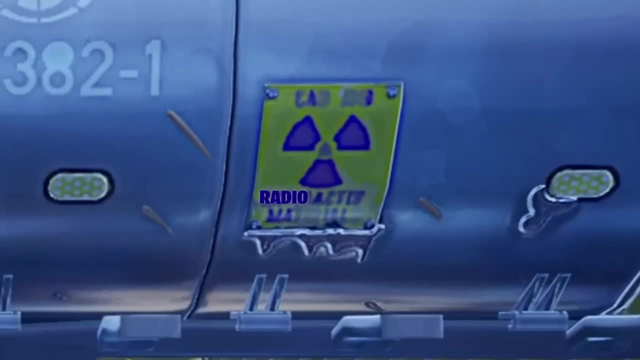 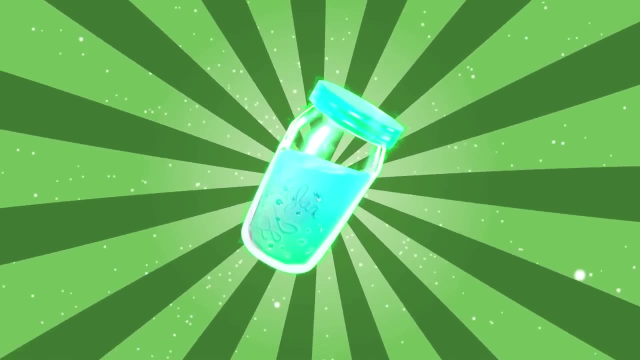 you'd see this little placard on the side of the truck that says Radioactive Material. The idea that Slurp Co would secretly be adding radioactive ingredients to their drinks does sound like the kind of thing an evil corporation would do, especially as we're covering it here on this. 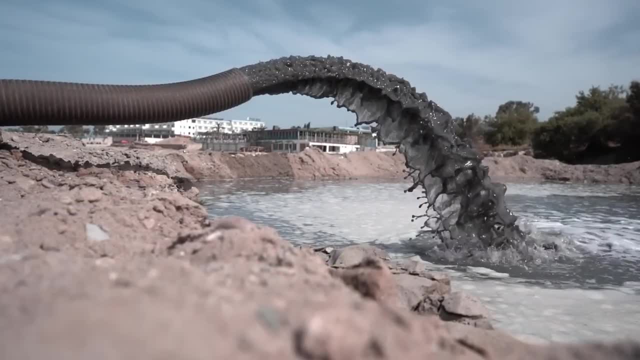 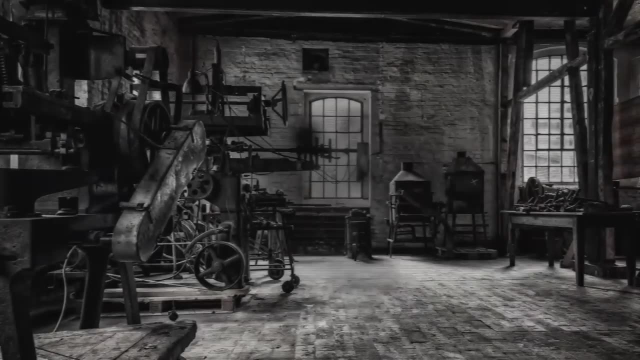 channel. But the funny thing is there are actually some real-world examples of companies doing exactly this, making their products radioactive. No, I'm not kidding. In the early 20th century, radioactivity had only recently been introduced and the idea of a slurping 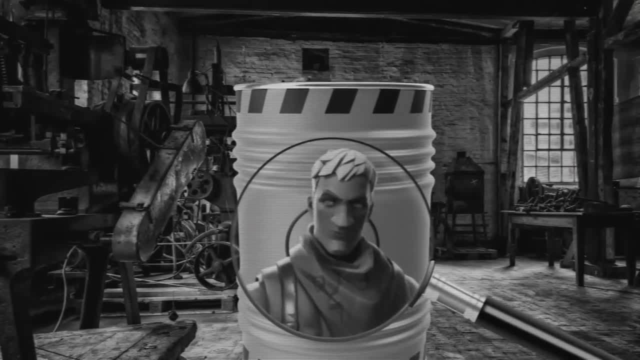 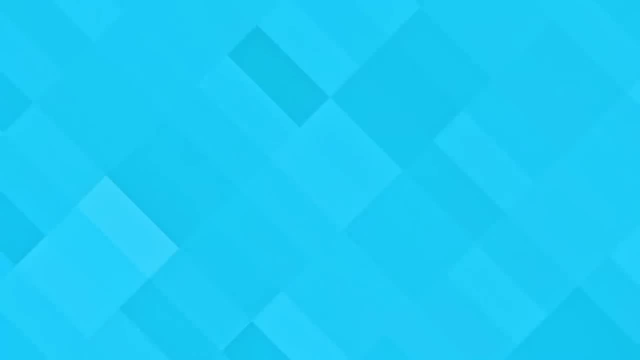 plant had been discovered, We're still decades away from understanding the long-term health effects of radiation exposure. All people really knew is that it contained a whole bunch of energy and that it glowed, So naturally, companies started shoving radioactive elements like 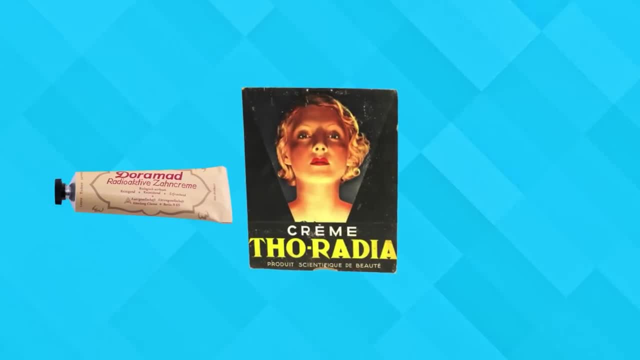 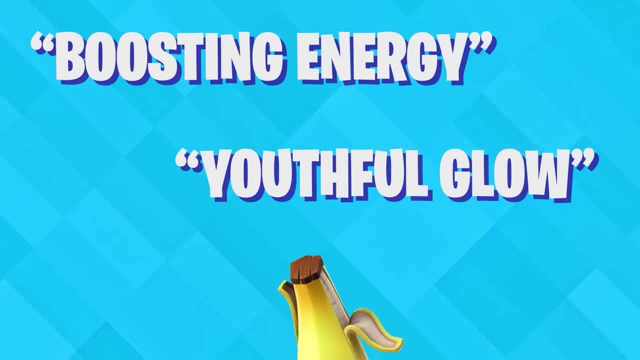 radium and thorium into anything they could think of, like makeup, toothpaste and even suppositories. Then they marketed them as boosting energy, giving you a youthful glow and improving your performance. But, as you can probably guess, that isn't what happened. One of the most 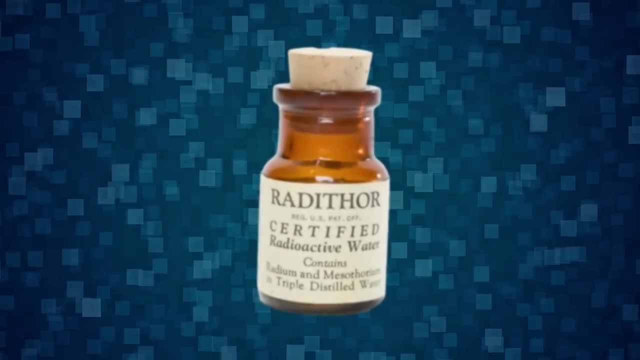 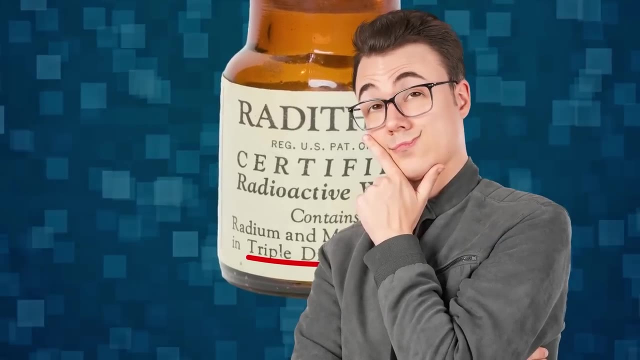 documented examples of this radioactive craze was for a product called Radithor. It was an energy drink that was basically radioactive radium mixed with- quote- triple distilled water. Oh good, wouldn't want any of those pesky impurities getting in my radioactive drink now, would we? 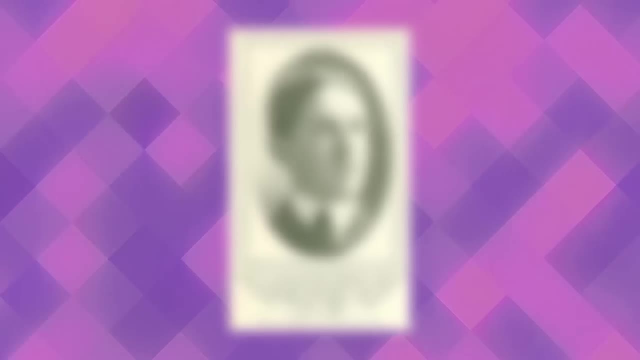 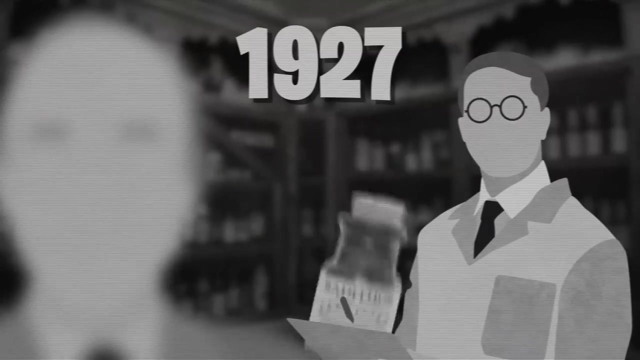 But one man was a big fan, businessman and semi-professional golfer, Eben Byers. In 1927, Byers hurt his arm after falling off a train bunk. His doctors ended up prescribing him Radithor. Oh, did I forget to mention this? stuff wasn't just an old-school gamer drink, It was. 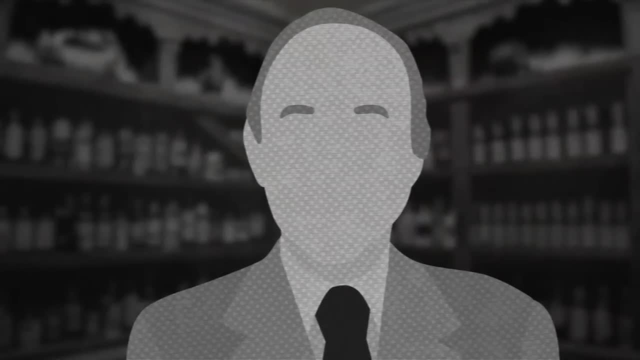 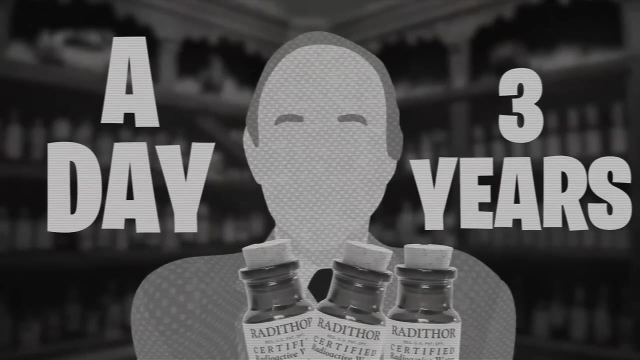 being prescribed as medicine. Byers said it made him feel toned up and would go on to drink an average of two to three bottles of Radithor a day for three years, Until, of course, it all came crashing down. Turns out that toned-up feeling was really his body falling apart, literally. 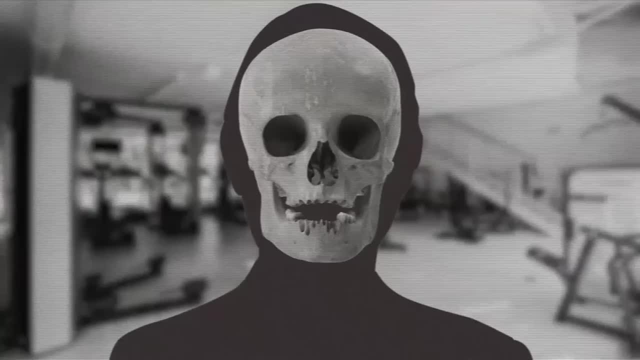 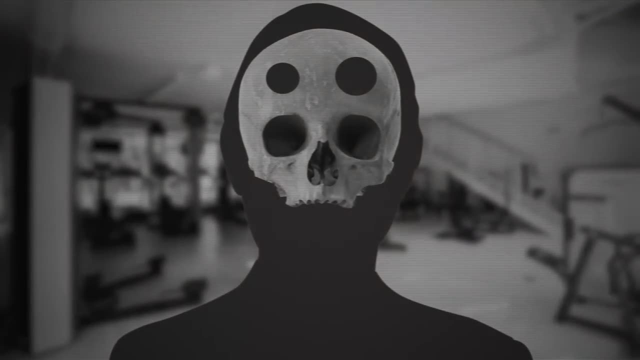 By 1931, he started to lose weight, his bones became brittle, his teeth fell out, holes started to form in his skull and eventually most of his bottom jaw had to be removed. He died in 1932 of multiple cancers. just five years after he died. 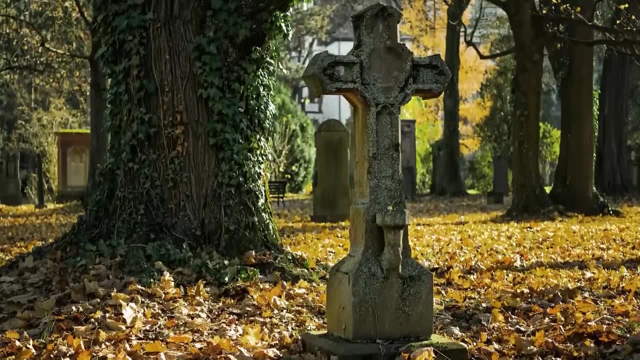 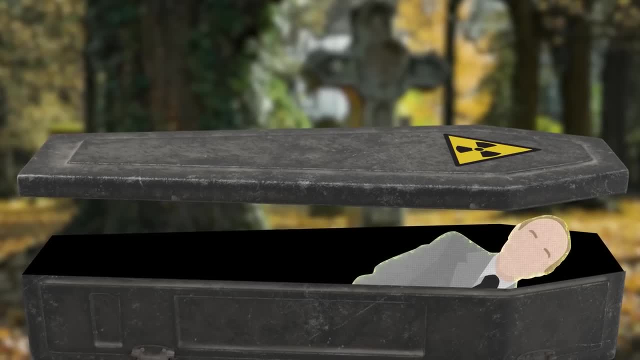 Five years after his first dose of Radithor, And then he had to be buried in a lead-lined coffin. Over three decades later, when his body was dug up for research, his corpse was still considered dangerously radioactive and likely will remain so forever. It was only after this and a few 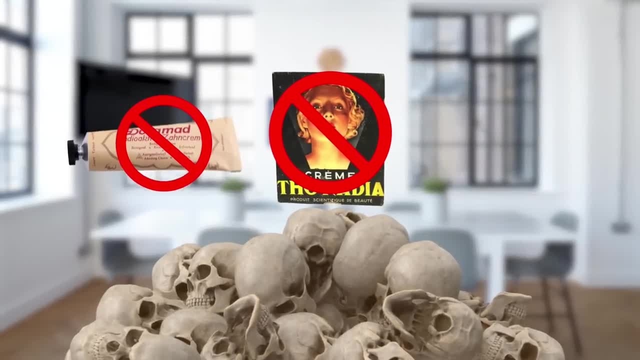 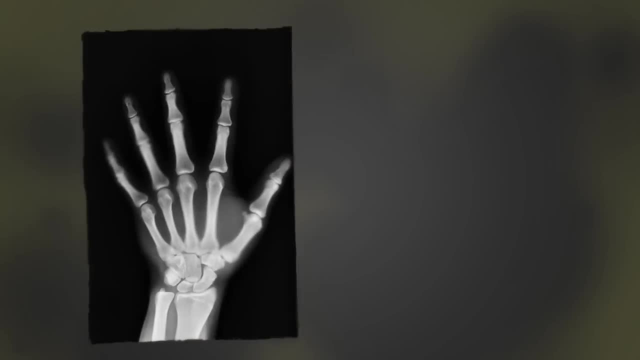 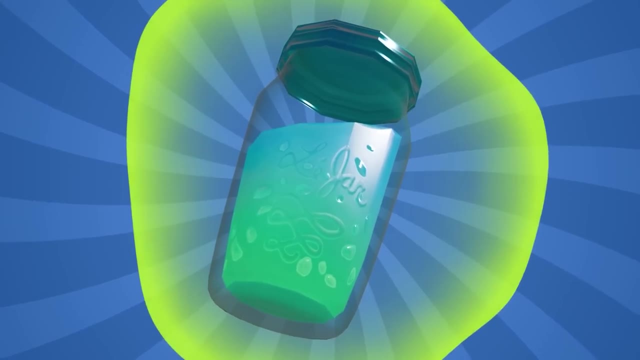 other tragedies that the FDA started cracking down and began regulating most radiation out of everyday products. Radiation is dangerous stuff and outside of niche medical applications like imaging and destroying cancer radiation serves absolutely no medical benefit. While it may be cool to think that the radioactive ingredients in slurp juice could, 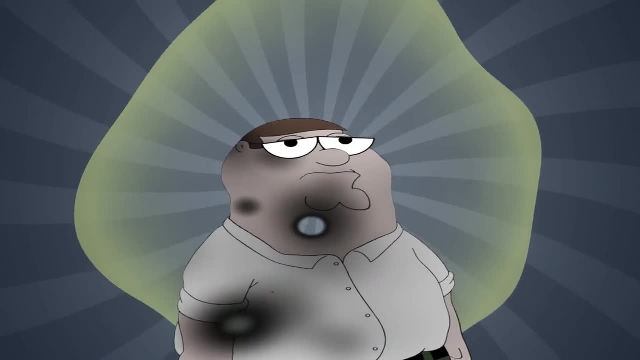 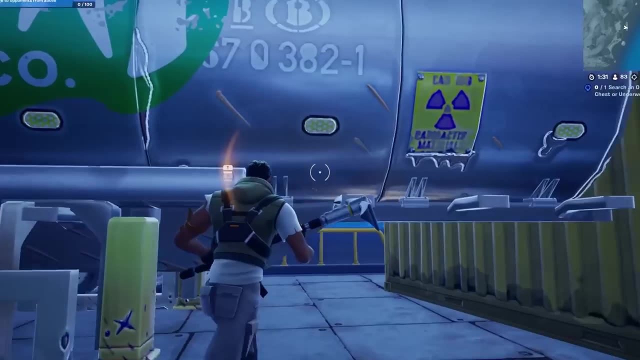 turn Peter Griffin into the Incredible Hulk. radiation doesn't really work like it does in the comics. It's less Bruce Banner and more Evan Byers. And actually, if you take a second look at those radioactive placards, you'll notice something. The lettering on those placards is old and worn. 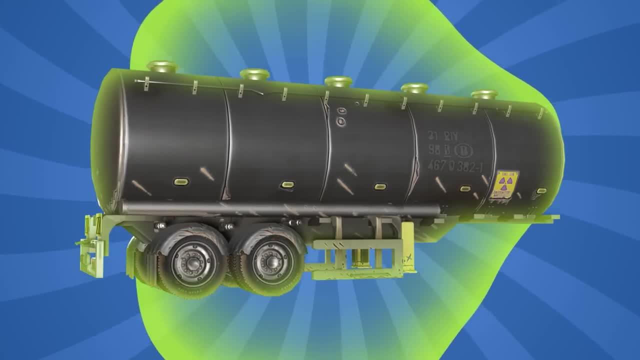 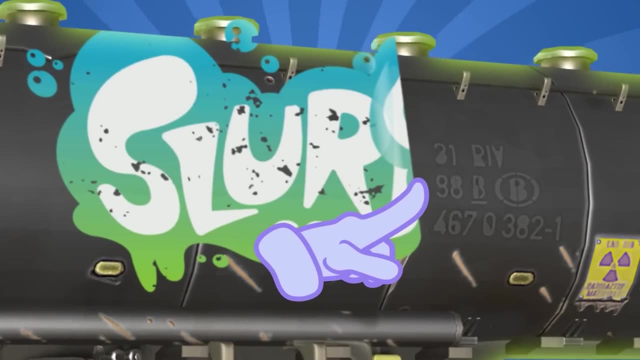 It seems to me that these trucks used to contain radioactive material but were bought and rebranded by SlurpCo somewhere down the line, which is why you can see other lettering peeking out from underneath the big beautiful slurp juice. 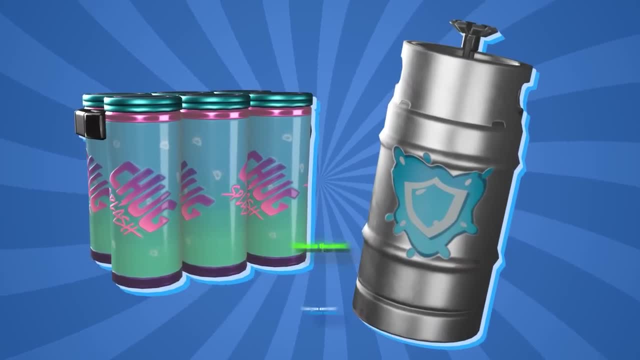 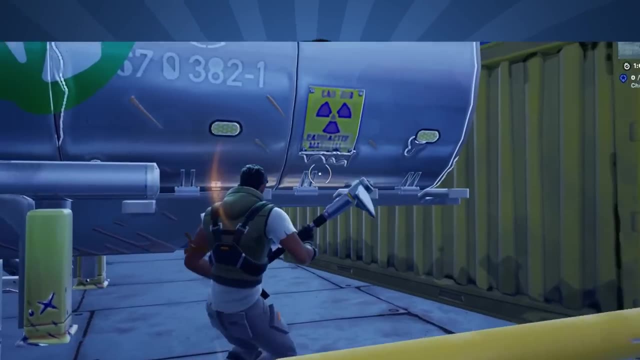 And it makes sense. I mean, none of their products are actively advertising the radioactive effects, like the products from the 1900s. and if they were trying to be sneaky about it you'd think they'd cover up the radioactive material sign on the side of their company. 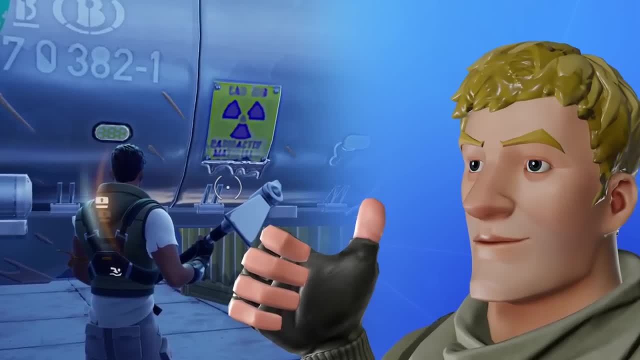 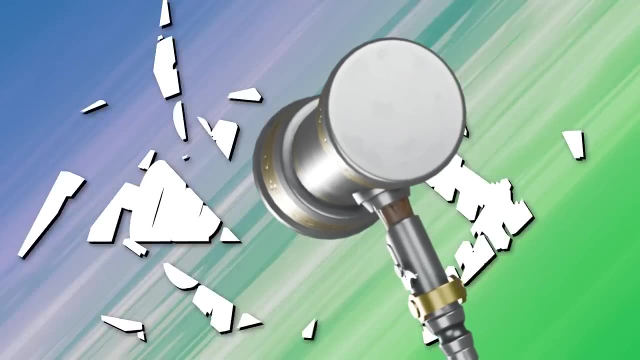 trucks That tied with the lack of missing jaws from our battle royales, and I think we can definitively say that slurp juice does not contain radioactive material. Okay, so if the game is no help, what real-world science is there that can help us to create? 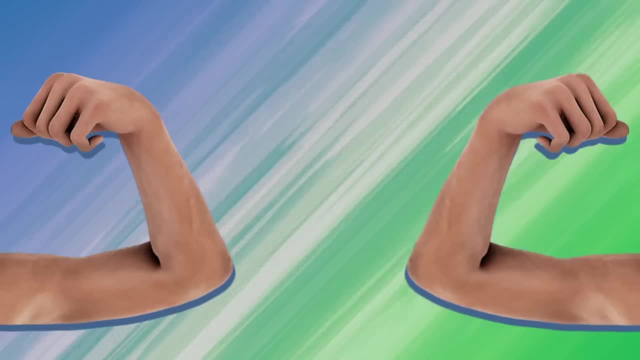 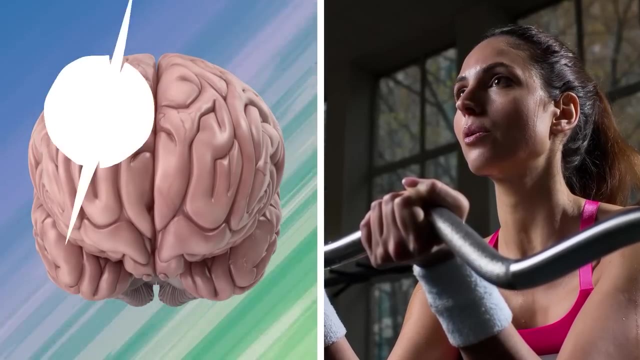 this beautiful blue slurp. I guess the first question really is: how and why do muscles actually get bigger? When you do any sort of strenuous activity, your brain sets off a cascade of metabolic processes across your body. It activates different genes to specifically protect you from the 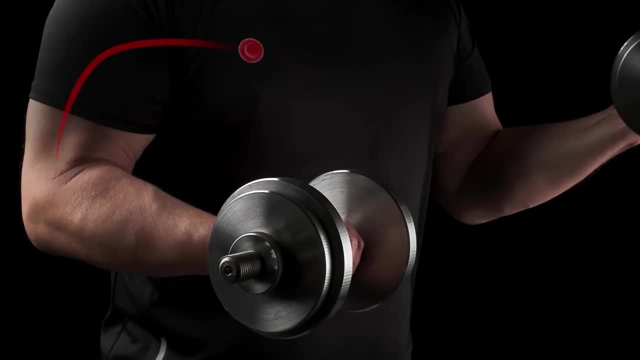 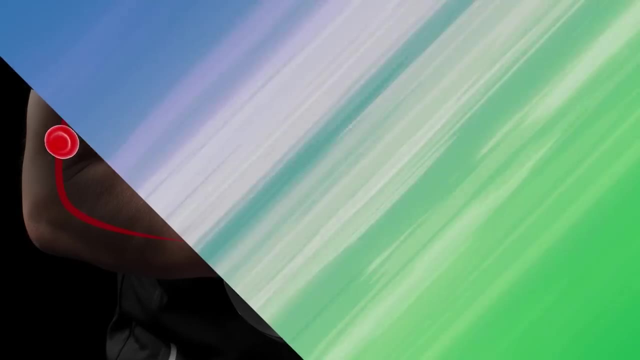 stresses of working out. For example, when you lift weights, your body starts funneling your blood towards the muscles and away from other parts of your body that aren't critical at that very moment, like your digestive system. After you're done pumping iron, you'll notice. 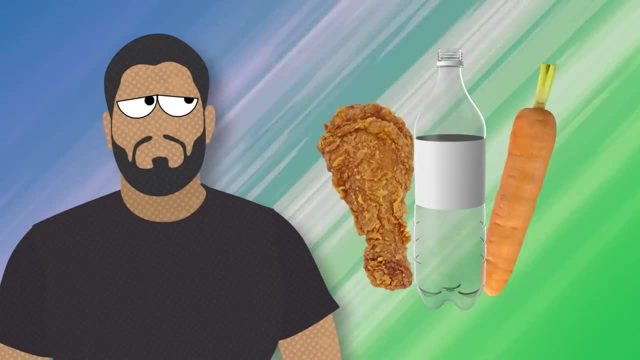 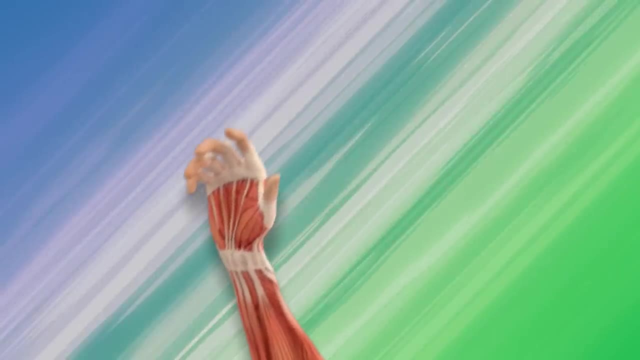 you feel a bit sore, That's because you've depleted your body of its critical nutrients and worked your muscles so hard that you've technically damaged them. Your body then reacts by repairing the damaged muscles, but this time making them even stronger than before. 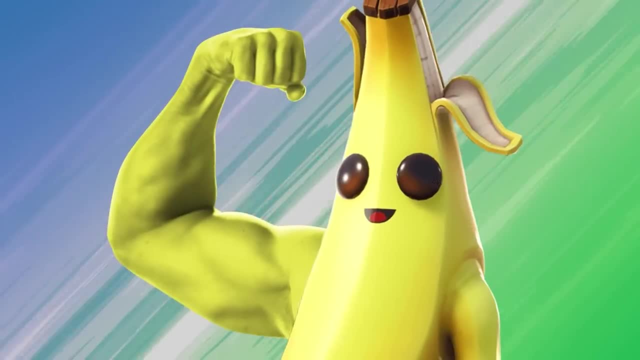 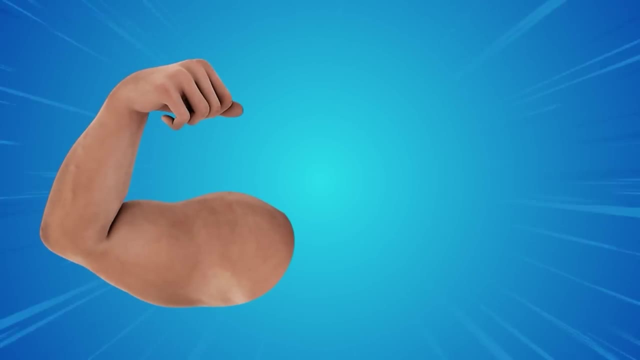 Over time, if you continue to work out that same muscle, it will eventually become jacked. So building muscle means you are also healing said muscles. Therefore, if we can focus on finding something that helps build muscle, we should get the healing factor thrown in. 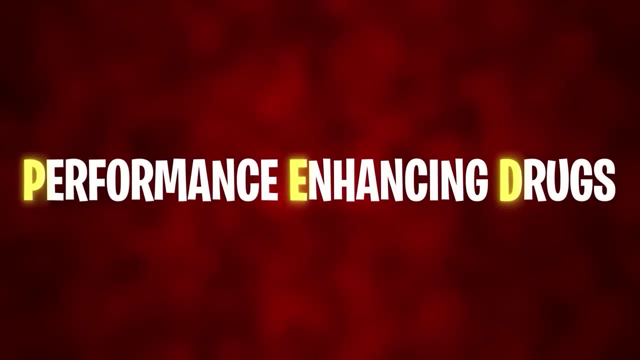 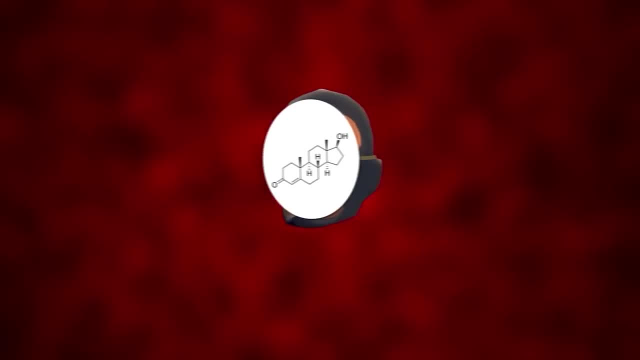 as a two-for-one. My first instinct was performance-enhancing drugs, or PEDs. Drugs like anabolic steroids allow athletes to illegally get swole fast. They do this by mimicking naturally occurring hormones in our body, like testosterone. Testosterone increases the production of muscle proteins, hence muscle growth and increased. 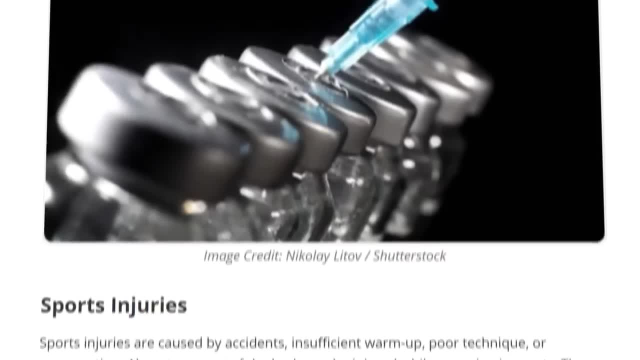 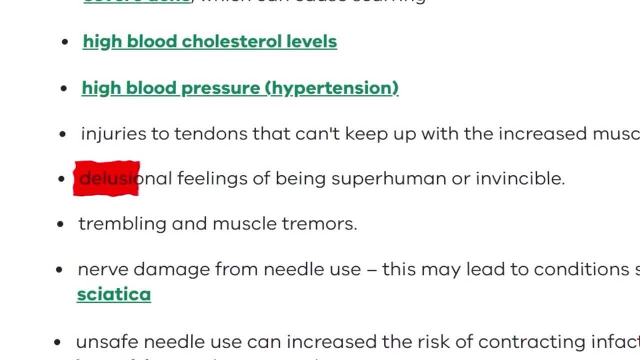 strength. It's not all illegal, though. Anabolic steroids can be used to help people recover from both muscle and bone injuries, strengthening them in the process. Plus, one of the side effects of steroid use is- quote- delusional feelings of being superhuman or invincible. And if 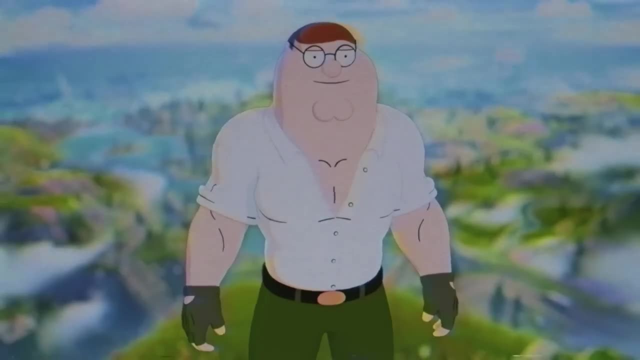 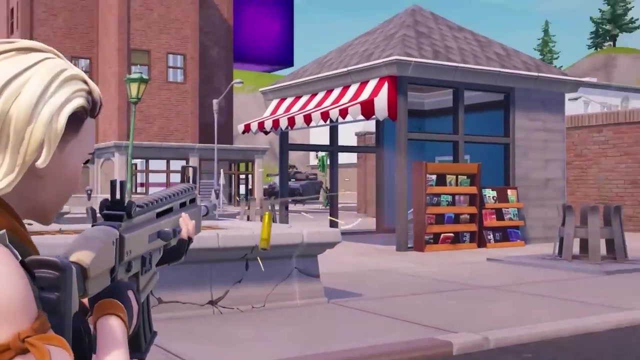 you take a look at Peter Griffin, I think that fits the bill quite nicely, Except when you then look at the other side effects. One of the long-term side effects of using steroids is muscle tremors, which isn't something you really want when you need to aim accurately. 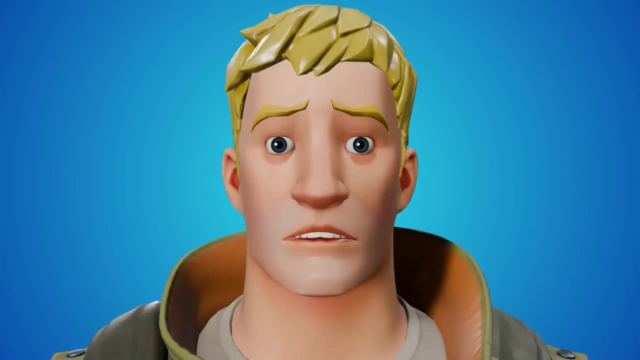 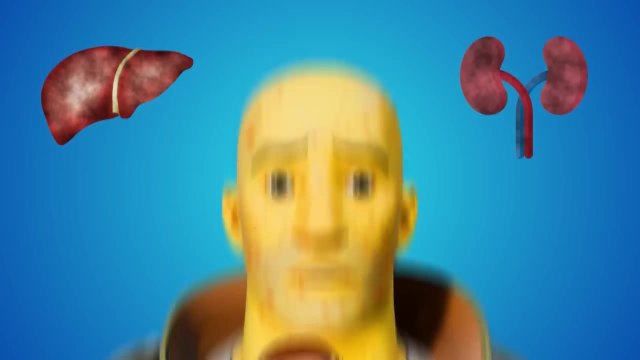 to take home the victory. Let's go through some more visually obvious side effects: Things like hair loss, severe acne and damage to your liver and kidneys, which can lead to things like jaundice making your skin turn yellow. That is not what we see of Peter. He looks like a Greek Adonis. 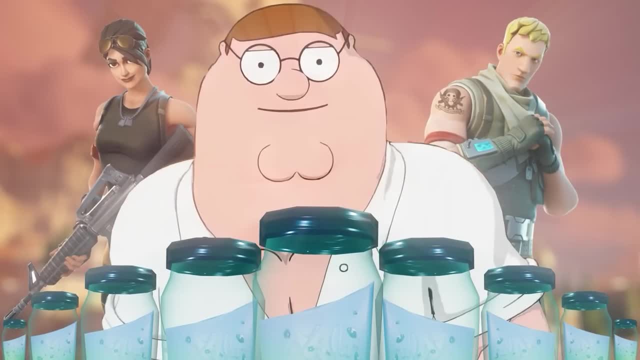 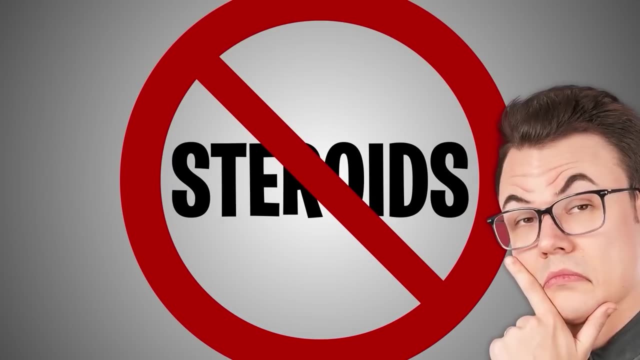 and our other Fortnite characters aren't looking bad either. Given how much these players are consuming during a game, it doesn't seem like these side effects are kicking in, which means it's likely not steroid use, which therefore means I have to keep looking. 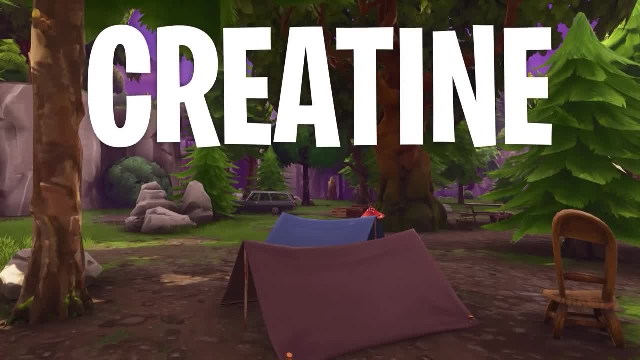 Naturally, I turn to the more natural option for bodybuilders: Creatine. This is typically found in things like fish and red meat. Instead of mimicking hormones, creatine is a very common side effect of the bodybuilder. Instead of mimicking hormones, creatine is a very common 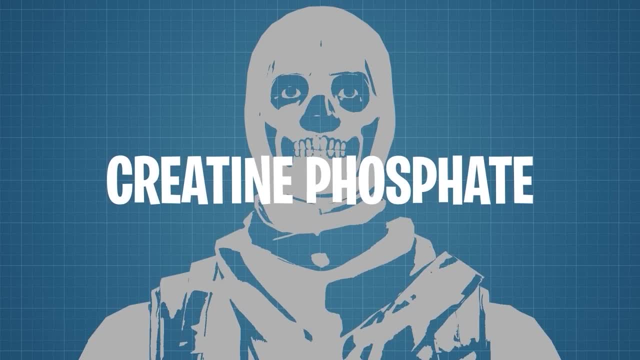 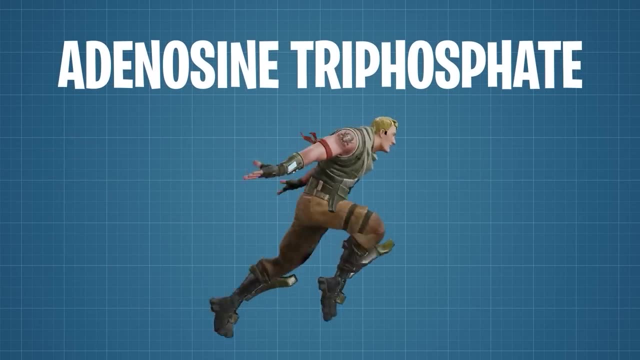 side effect of the bodybuilder. Creatine goes straight to your skeletal muscles and is converted into creatine phosphate, which then helps with the creation of adenosine triphosphate, an energy source for your cells. Basically, it allows you to exercise for longer. 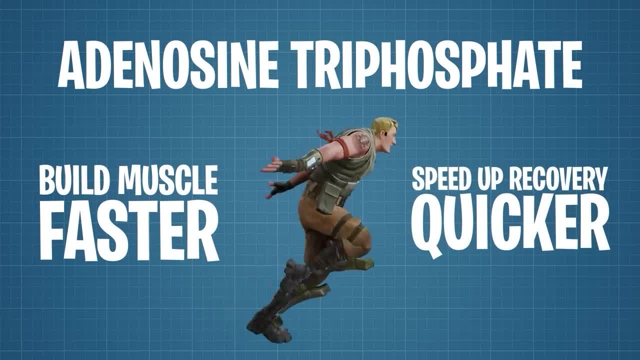 therefore helping you build muscle faster and helping to speed up the recovery of those muscles. Not to mention that it's currently being studied to see if it can potentially treat things like congestive heart failure, Parkinson's and fibromyalgia. so the healing. 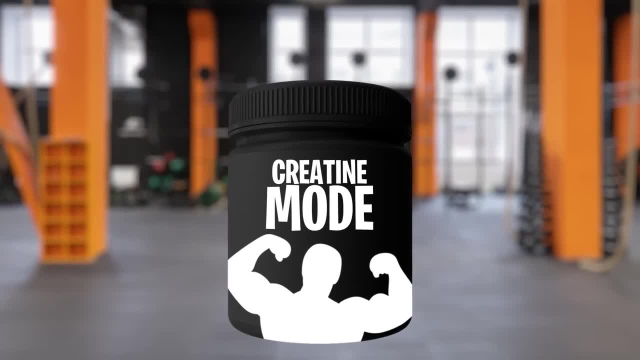 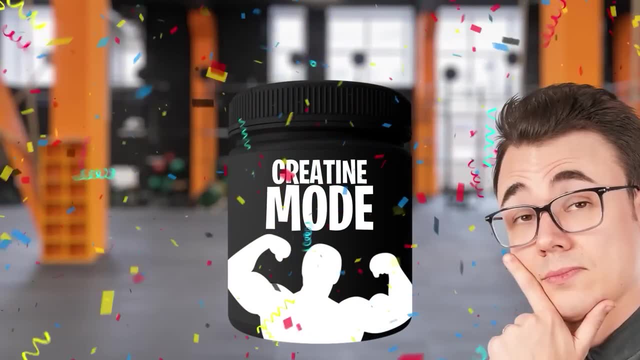 factor is definitely there. Finally, creatine is typically sold in a powdered form, which makes it easy for Slurp Co to sneak it into your juice. It seems like we have a winner- lack of negative side effects, but it's still not a perfect fit. Both creatine and 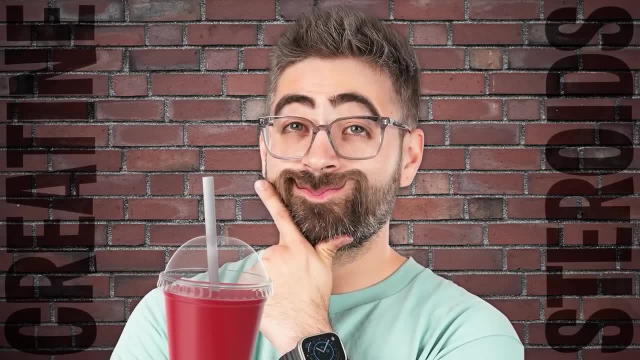 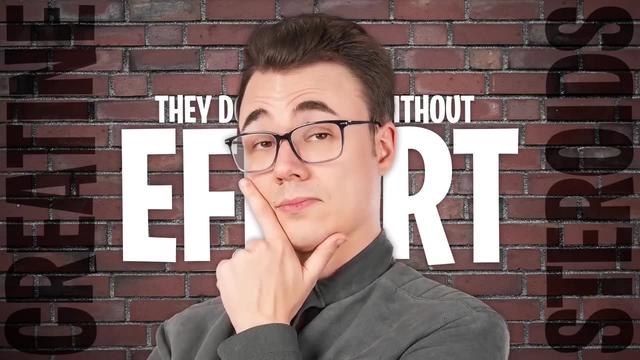 steroids run into the same problem we did earlier, Much like the nutritious juice that Santi laid out for us. these things don't work without putting in some level of effort, And it was at this point that I was basically ready to give up. There just didn't seem. 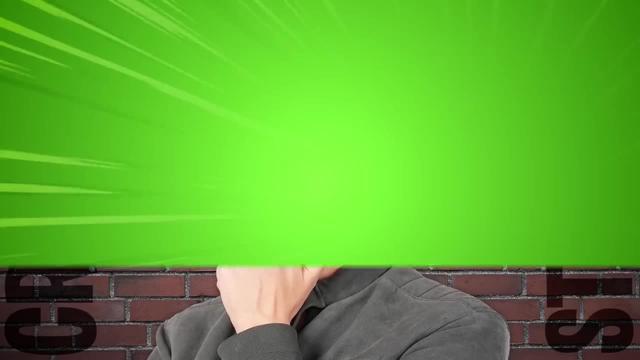 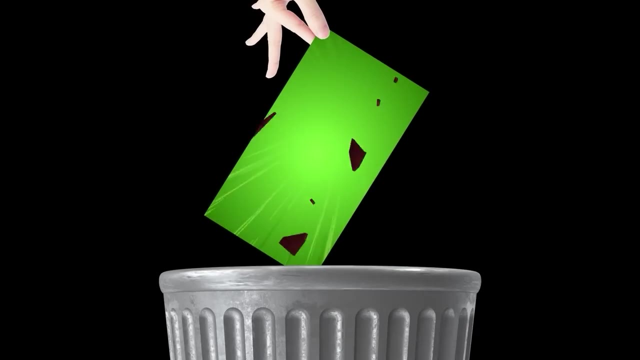 to be any way to grow your muscles without putting in the work. Epic Games had specifically designed the most unscientific item possible, and so my couch potato dreams were shattered, and I was this close to binning the entire episode. That was until I found this At the 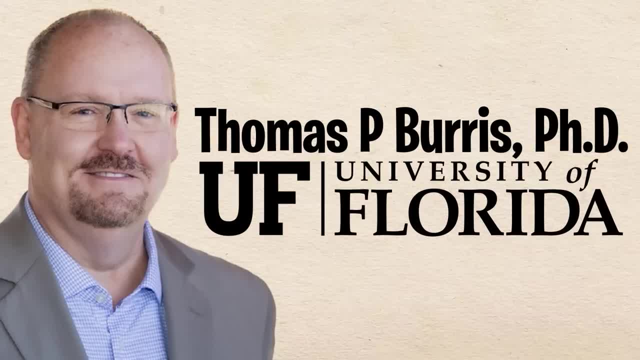 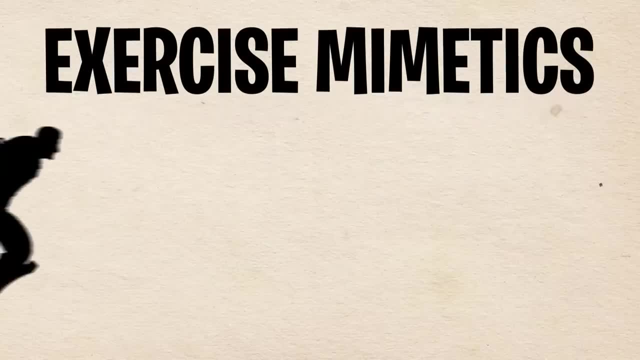 end of the video, a group of scientists led by Dr Thomas P Burrus from the University of Florida announced some promising results on an experimental new drug. This drug is part of a class of compounds called exercise mimetics. Basically, these are compounds that 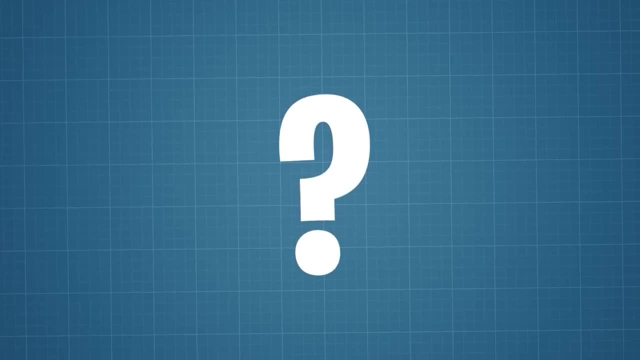 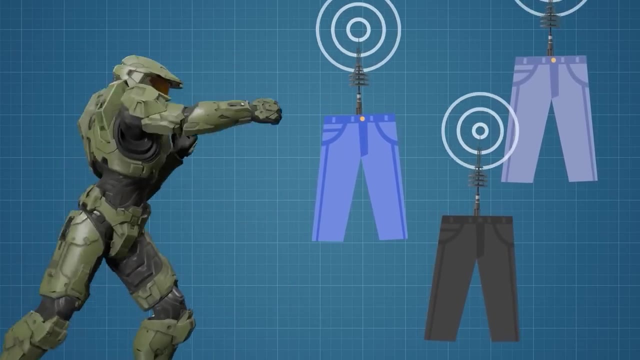 mimic the effect of exercise without having to exercise. How does it work? Well, earlier we mentioned that when you exercise, your body activates different genes. That happens because those genes have receptors that bind to different proteins. One of those receptors is known as an estrogen-related receptor, or ERR. Fun fact has nothing to do with estrogen. 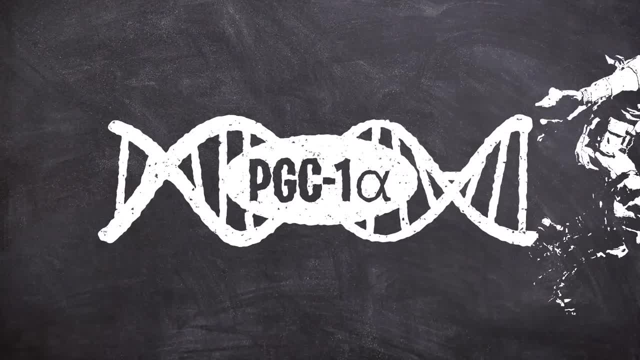 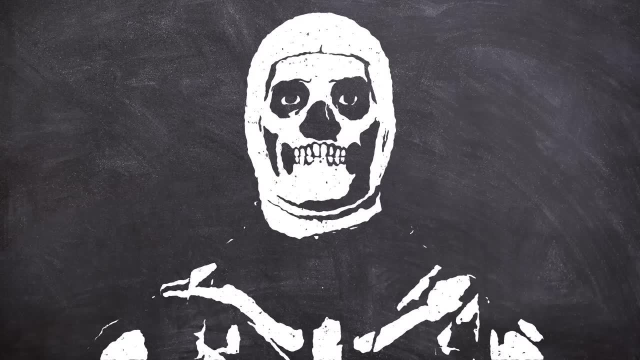 the hormone, The more you know, I guess. But when you exercise, your body releases a protein called PGC-1-alpha and that binds to a lot of receptors in your body, including ERR, which then stimulates the production of skeletal muscle fibers. However, PGC-1-alpha isn't specifically meant for ERR. In fact, 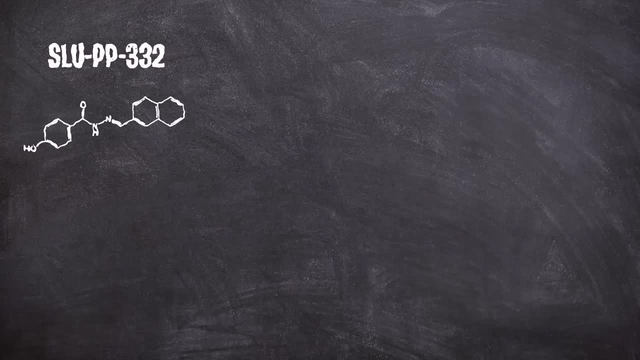 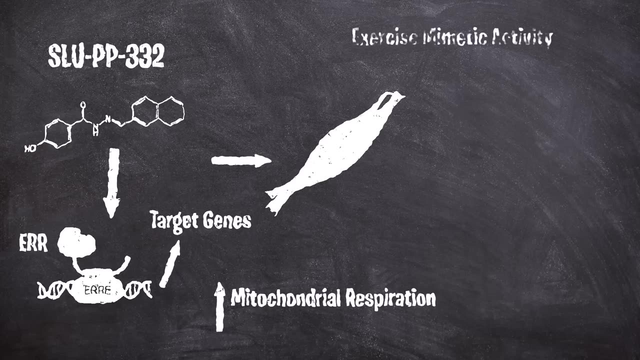 no protein is, which is where this new drug comes in. It was designed specifically to bind to those estrogen-related receptors in place of PGC-1-alpha, activating the genes to produce skeletal muscle fibers and therefore tricking your body into thinking the muscles. 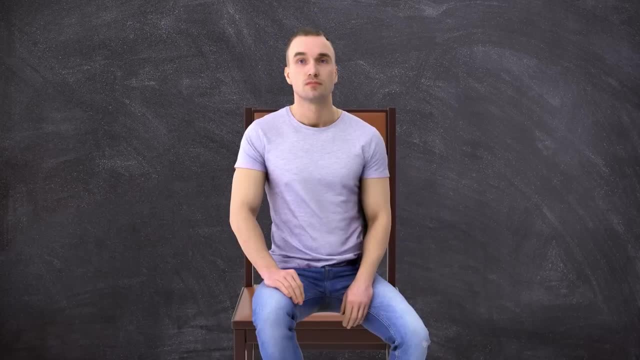 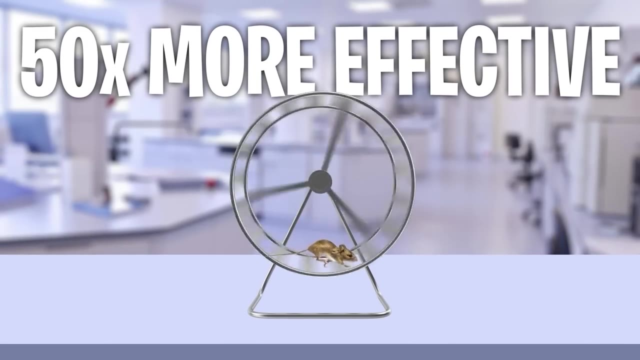 are damaged and need repairing And so building muscle, All without having to leave your chair. During trials on mice, they found that it was actually 50 times more effective than traditional training, with those given the new drug being able to run 50% further than. 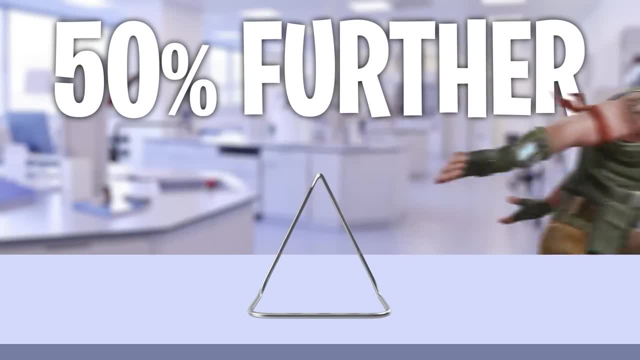 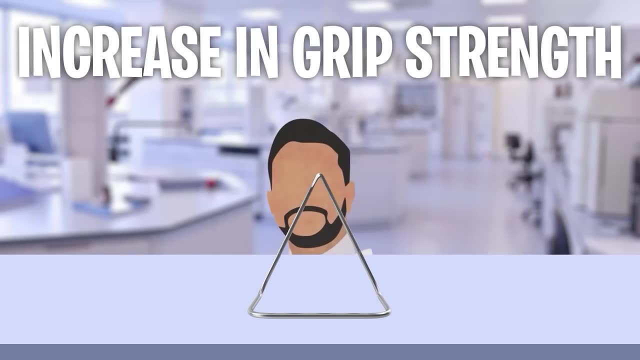 those who weren't Considering that a player needs to run for miles in a 20 minute game. that sounds like it would be pretty useful. You know what else the scientists found during the experiment, outside of the increased muscles and healing properties? An increase in grip. 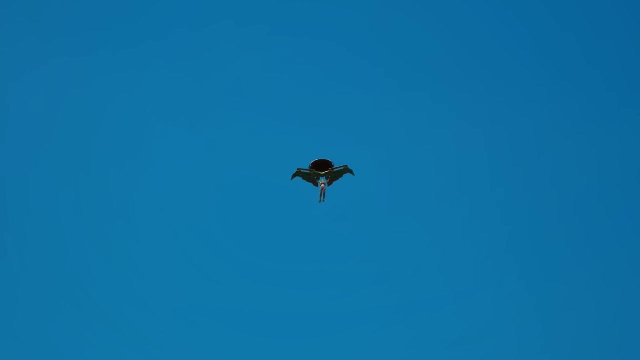 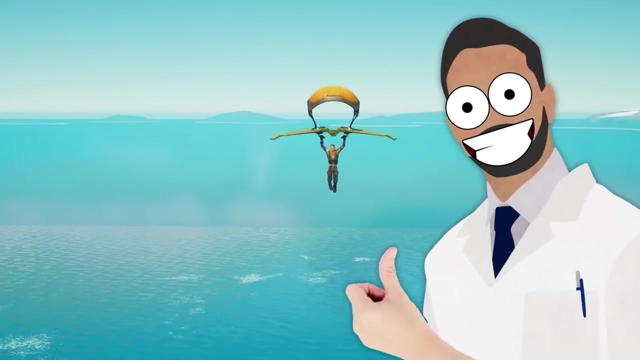 strength, Which, when you remember that a player needs to paraglide all the way from the battle bus to the island, seems like a critical advantage. And what's great about all of this so far is that scientists haven't noticed any long-lasting 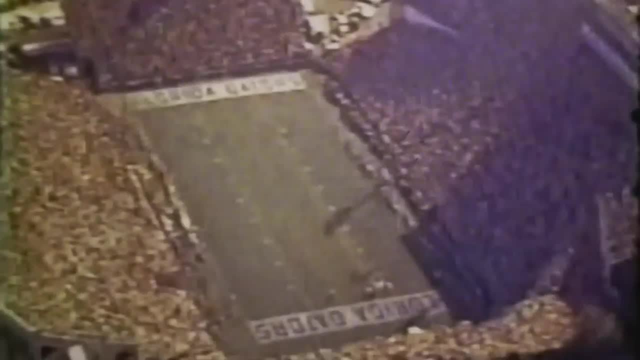 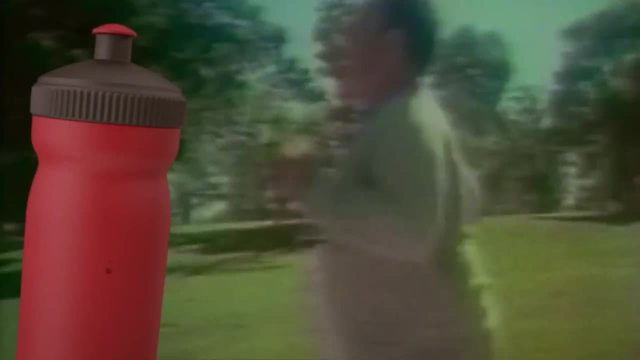 negative side effects. It's also worth noting that the university doing these experiments is the same university that made another sports beverage innovation. back in the 1960s, They created a sports drink that provided electrolytes and other nutrients to help aid the performance of their football team, the Gators. Of course, this drink would then go on to be known as. 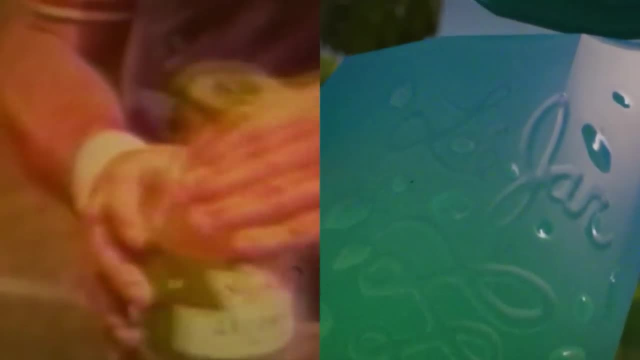 Gatorade, Famous for its bright colors, including blue, and if you take a look at the original bottle, it does look an awful lot like slurp juice, doesn't it? And if you take a look at the original bottle, it does look an awful lot like slurp juice. 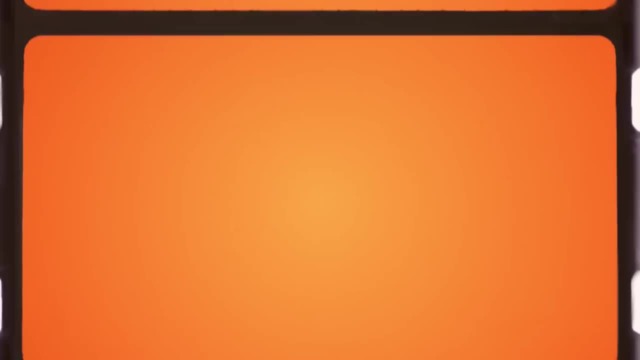 doesn't it? And if you take a look at the original bottle, it does look an awful lot like slurp juice. but the absolute cherry on top of all of this is the drug's name. the absolute cherry on top of all of this is the drug's name. 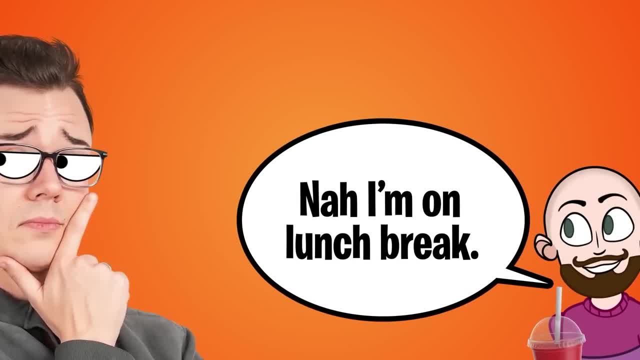 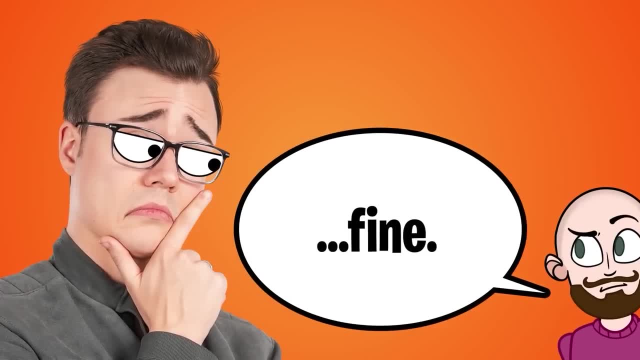 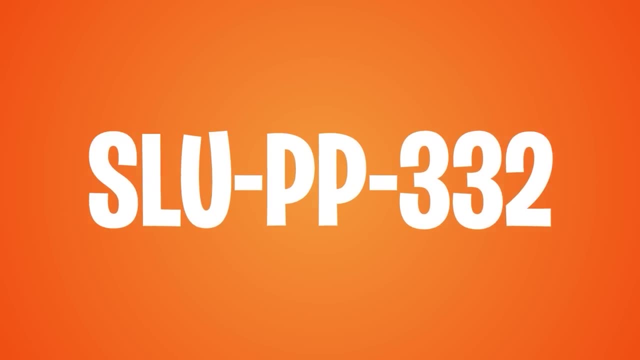 YOSEY Drum roll. please, Come on, man. this is this is my first one- like: can we maybe just put a bit of effort into this, Please? I'll bring you chocolate from the UK, Please. Thank you. The name of this drug is SLUPP332.. I mean, you see it right, Come on. It's basically. 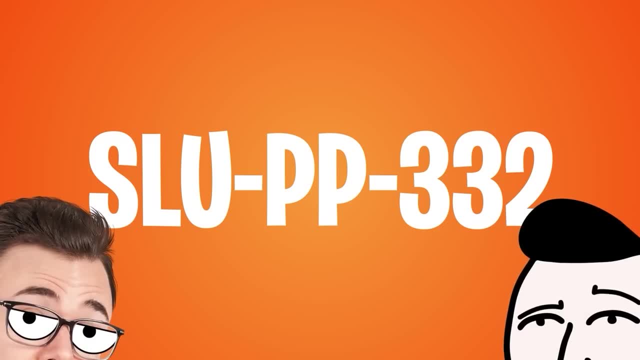 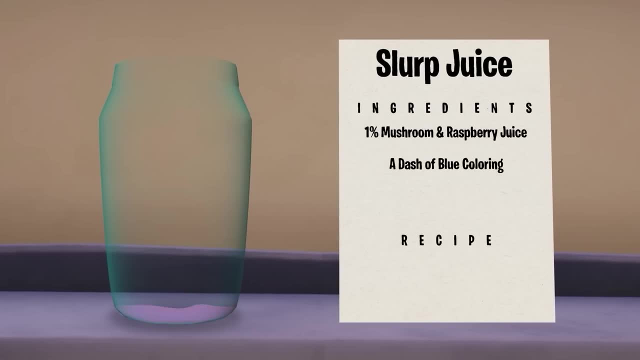 one line away from just being called Slurp Editor. can we fix that in post, Thank you. So there you have it, The true recipe for slurp juice: 1% mushroom and raspberry juice. maybe a dash of blue colouring to make it feel like a healthy sports drink. 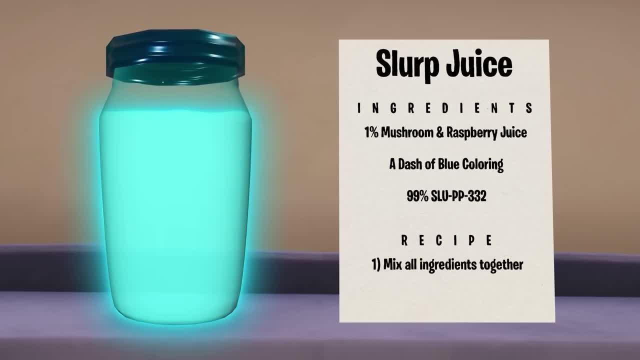 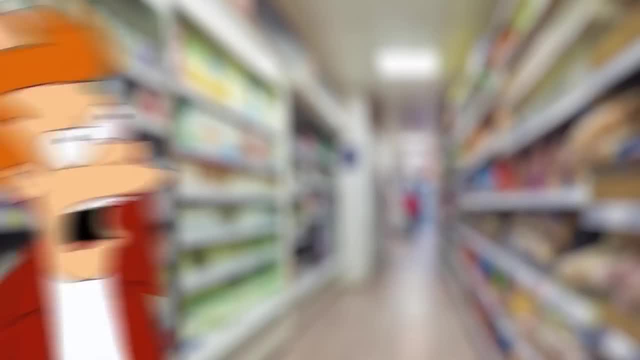 and the rest is all. SLU-PP332,, an experimental drug designed to help you gain muscle without lifting a finger. Perfect for people like me stuck behind a desk all day writing theories. Of course, right now you can't just go out and buy slurp. It's still very much in the early testing phase. It needs to be trialled and refined before it ever gets into a person's body Because, while early results show that it doesn't have long-term side effects in mice, even that only looks at the effects after a month or so. 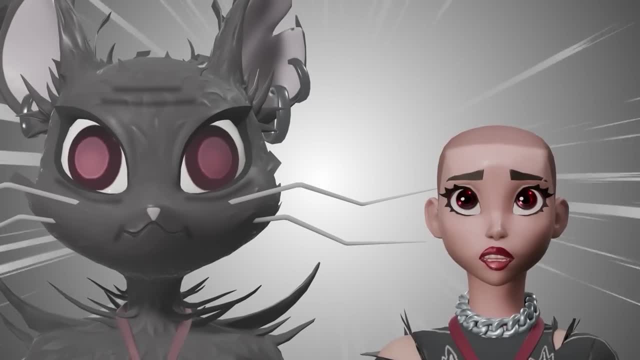 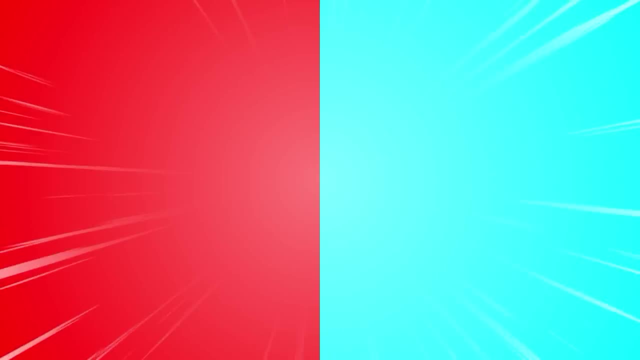 Who's to say that taking the drug for longer or when it's trialled on humans doesn't cause some kind of unforeseen side effects. However, this clearly hasn't stopped Slurp Co from releasing the product anyway. That's why, unlike other juices that you find in the game, like Slap Juice and Guzzle Juice, 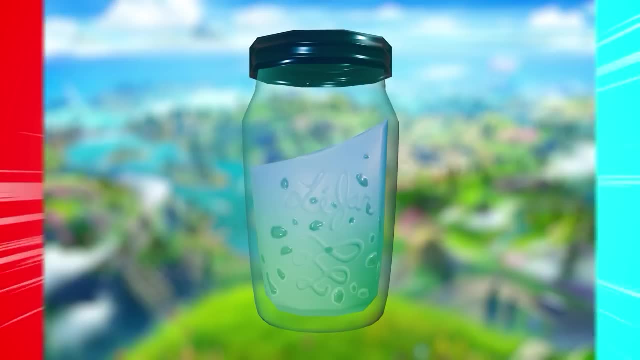 which come in more traditional consumer packaging. like we see in our world, Slurp Juice comes in an unlabelled mason jar. It's the kind of jar you buy at a craft store, not the one you'd use to mass market a product. 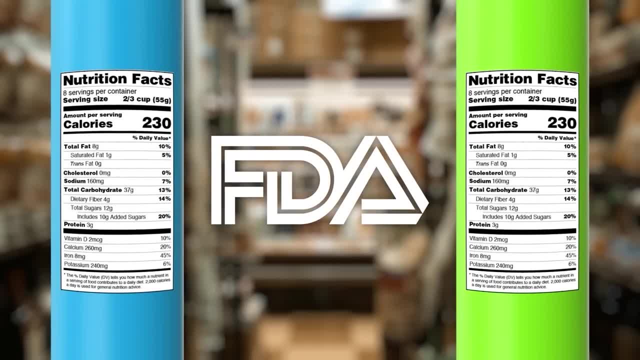 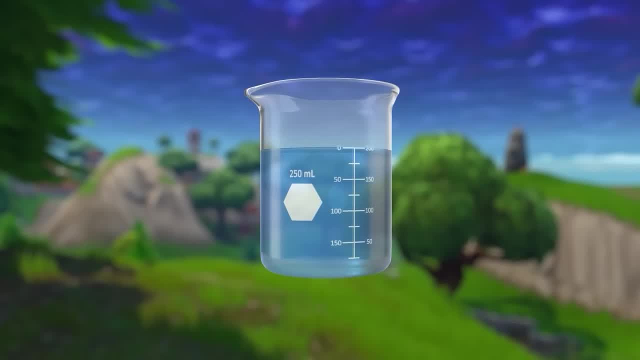 All those labels you see on food and medicines. That has to be there as part of the food and drug administration's approval process to let you know what the side effects and health risks are for anything you're consuming. But we don't know the side effects of Slurp Juice. 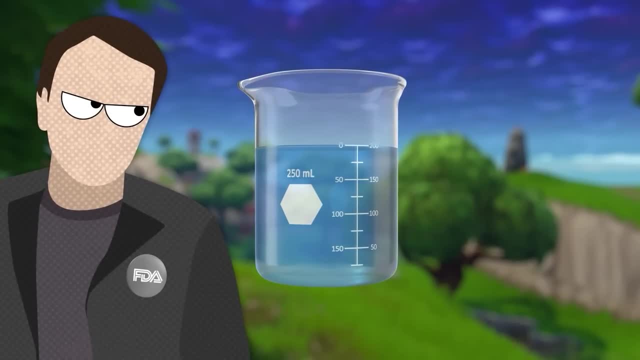 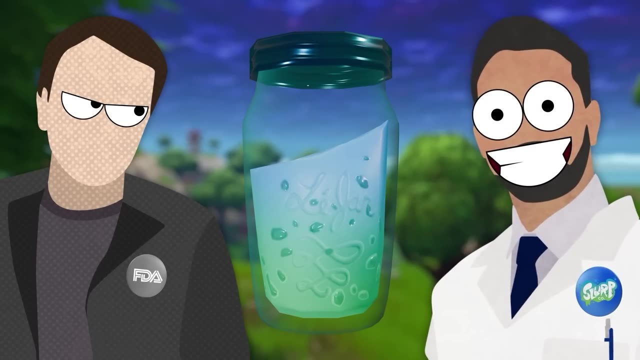 which would be an immediate red flag for the FDA, And that is why it's given out in unlabelled mason jars. We're being told it's just raspberry and mushroom juice that will give you a little extra boost to keep fighting, when in reality our players are a series of guinea pigs. 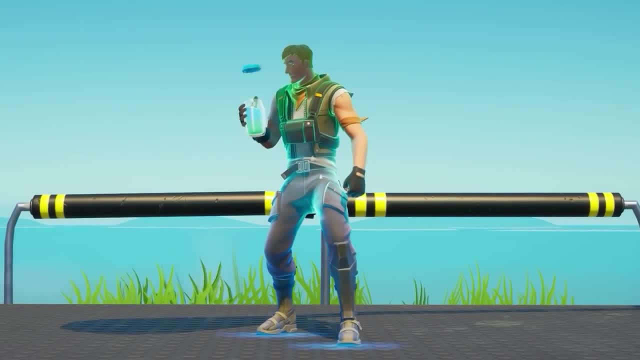 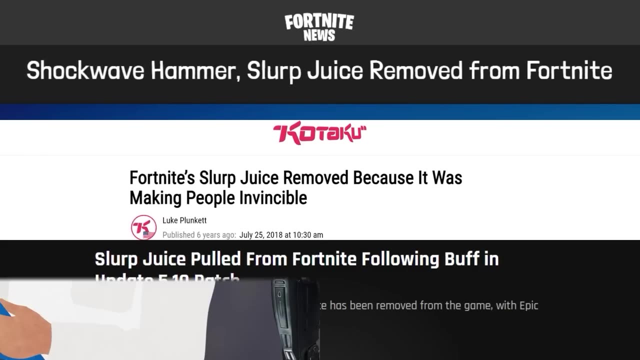 testing out a brand new experimental drug without any approval, completely ignorant to any potential slurpy side effects, And considering the fact that Slurp Juice has been removed from the game time and time again, my guess is they either got found out or those trials didn't go so well. 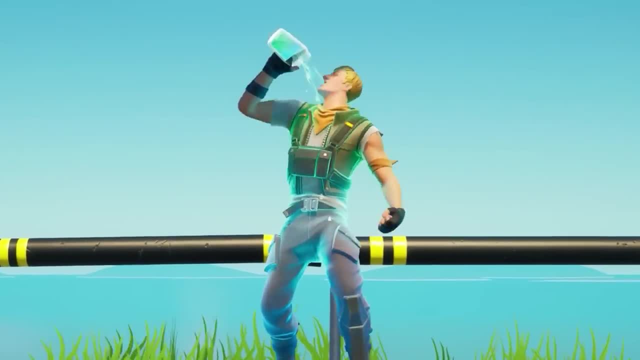 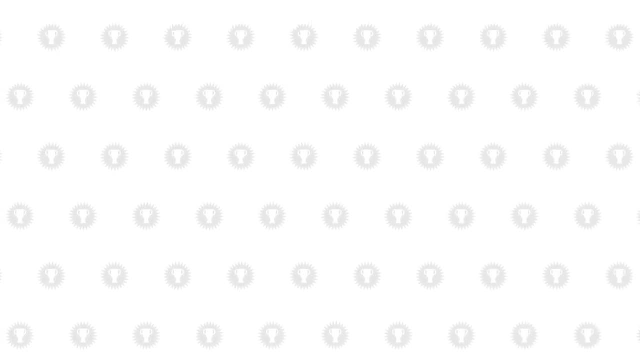 Maybe I'll just stick to the gym. But hey, that's just a theory, A game theory. Thanks for watching. Hey, remember that loud, annoying guy who rudely interrupted me earlier. Turns out he does more than just pester me. 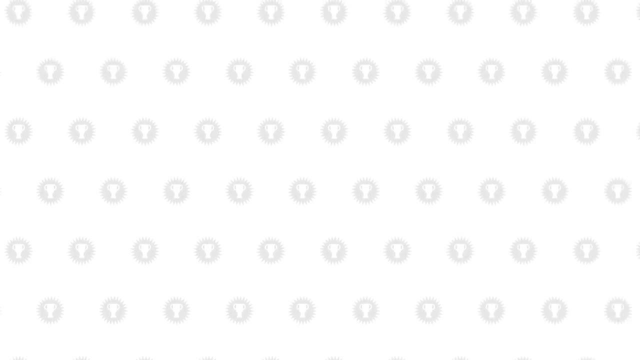 Over on Food Theory, Santi broke down what it takes to make the perfect spicy chicken sandwich. That link is over on the left and if you do click it, let him know. Tom sent you. He'll hate it If you prefer another Fortnite theory.